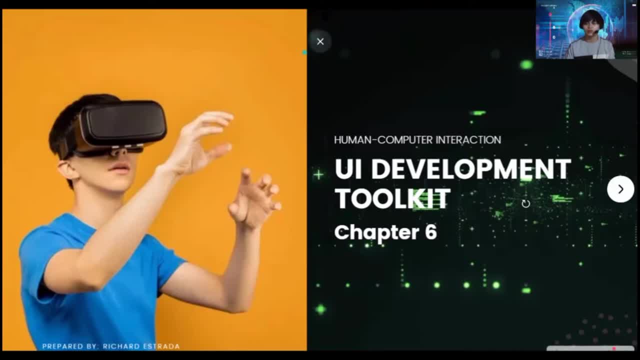 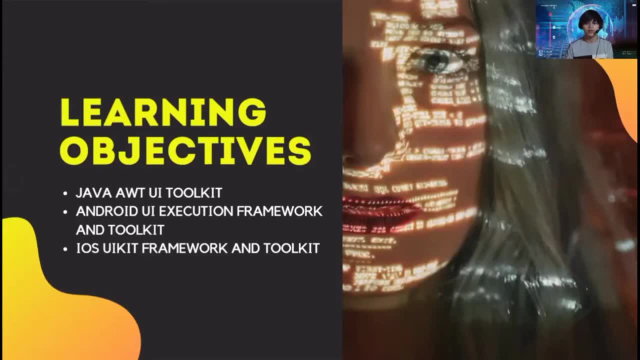 So let's start with our first slide. Okay, the learning objectives. Okay. so for this chapter we will be discussing about the Java out UI toolkit, the Android UI execution framework and toolkit, the iOS UI kit framework and toolkit. So all about toolkits or different kits, Okay. 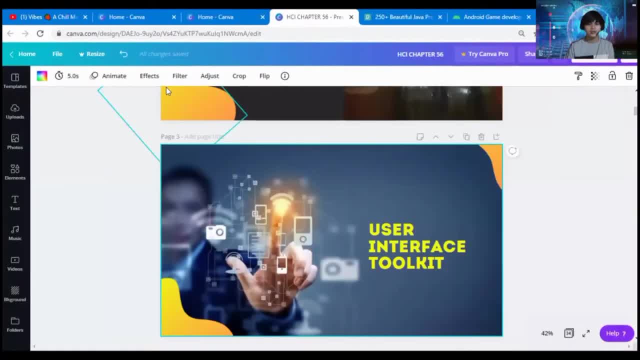 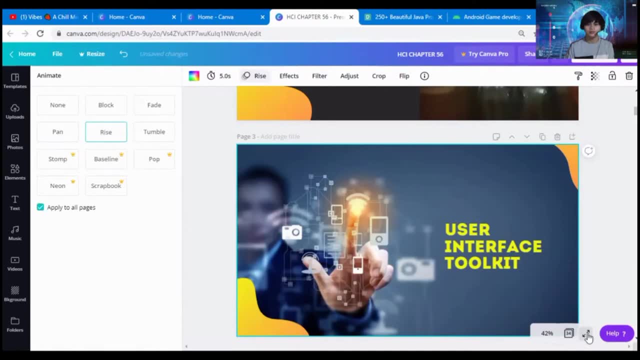 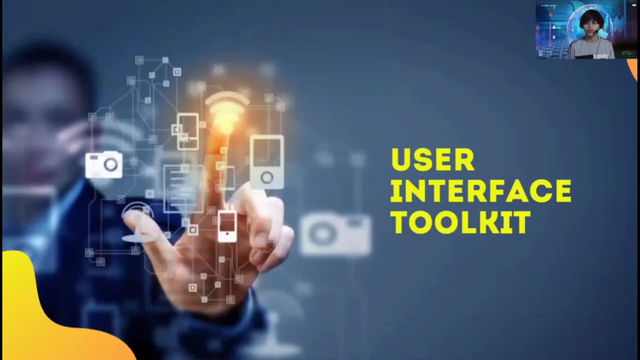 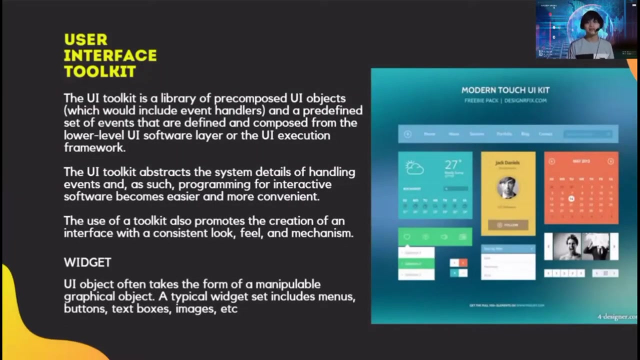 Wait, let's add some animations. Okay, So let's discuss first the user interface toolkit or the UI toolkit. So what is a UI toolkit? Okay, So the UI toolkit is a library, Again, a library of pre-composed UI objects, which would include events, objects and objects. So the UI toolkit is a. 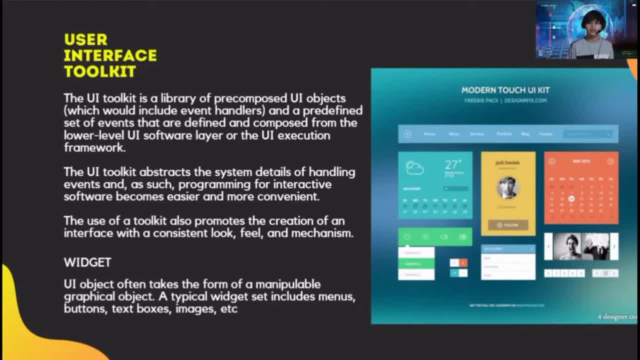 set of events that are defined and composed from the lower level UI software layer or the UI execution framework. Okay, so the UI toolkit abstracts the system's details of handling events And, as such, programming for interactive software becomes easier and more convenient. 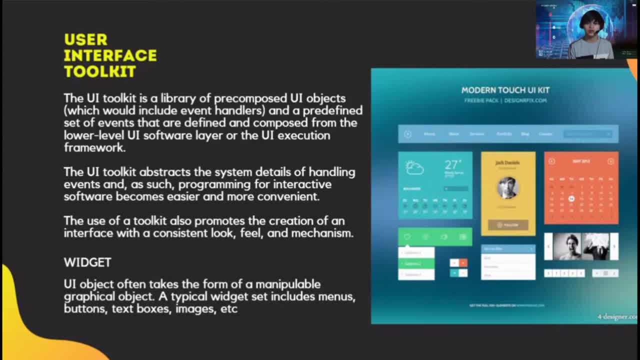 So the use of a toolkit is also promotes the creation of an interface with a consistent look, feel and mechanism. So it's actually a library in order for you to produce, you know, buttons, stacks, images, inputs, etc. And there is what. 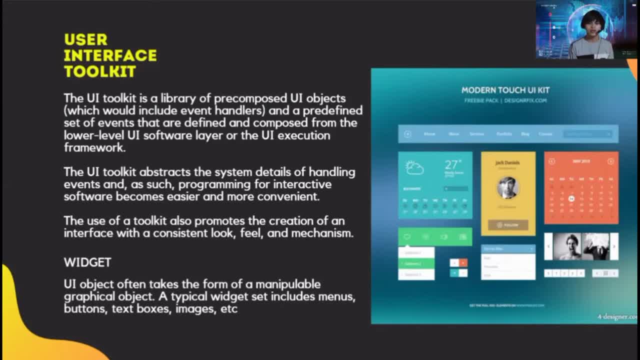 we call widgets in a user interface toolkit, So it is a UI object. often takes the form of a manipulable graphical object. Okay, A typical widget is Widgets set includes menus, we also have buttons, we also have text boxes and then images, inputs, etc. and a lot more and everything that you have on your design. okay, 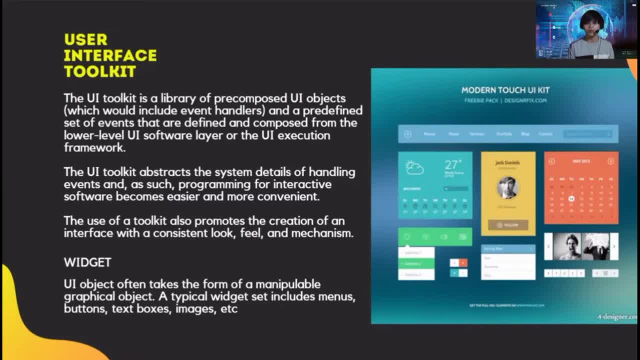 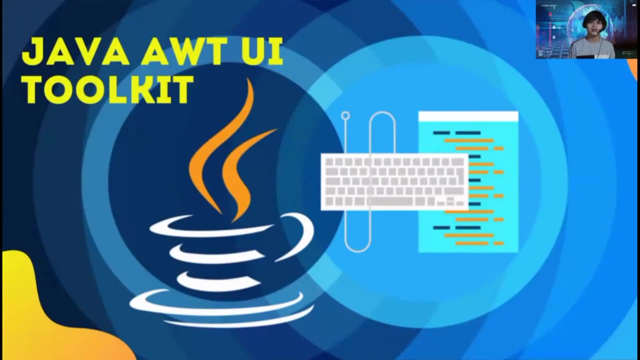 So that is a toolkit. Again, it is a library of pre-composed UI objects, So we're going to help programmers or you to build a really great application. okay, So first let's discuss the Java Out UI Toolkit. 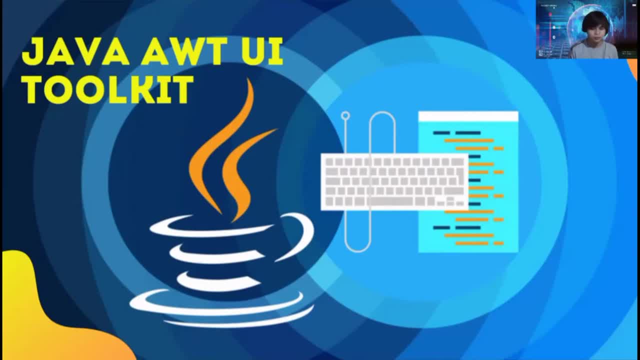 So Java is a programming language and there are a lot of programming languages that we can use when we want to develop Android applications, iOS applications, web applications and, yeah, and a lot more, But for this chapter, we will only be dealing with the Java programming language. 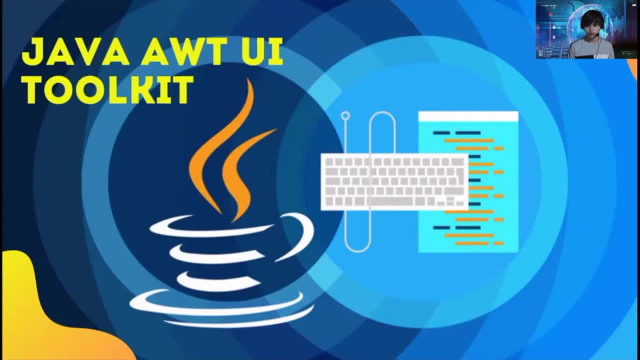 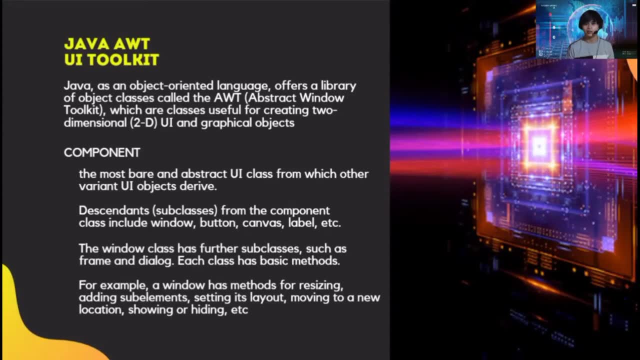 So we're going to discuss the Java Out UI Toolkit. Okay, again, Java is an object-oriented language, So we're going to discuss about Java. We're just going to get the concept on. how are we going to develop using Java programming language. okay, 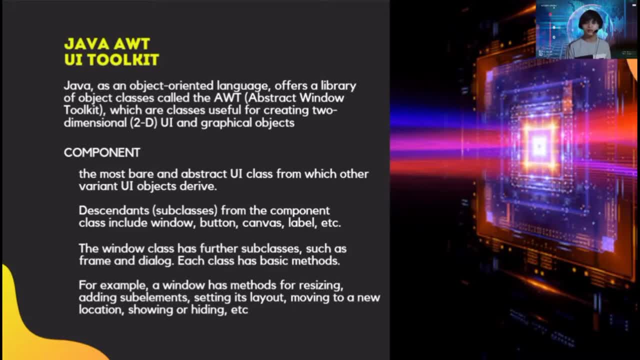 So it offers a library of object classes. called Out Out means abstract window toolkit. okay, Which are classes that are built with an object, are classes useful for creating two-dimensional or 2d ui in graphical objects. so in java we use this. 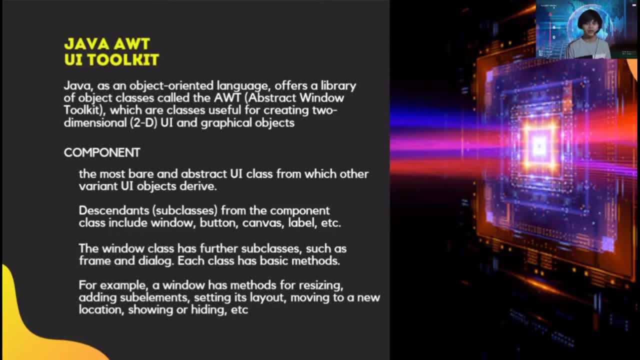 out the abstract window toolkit, okay, and out has this what we called components. okay, sorry, let me drink first, since you know guys. so, um, the most bare and abstract ui class from which other variant ui objects derive, okay, descendants or the subclasses from the component, includes window button, canvas and label. so the 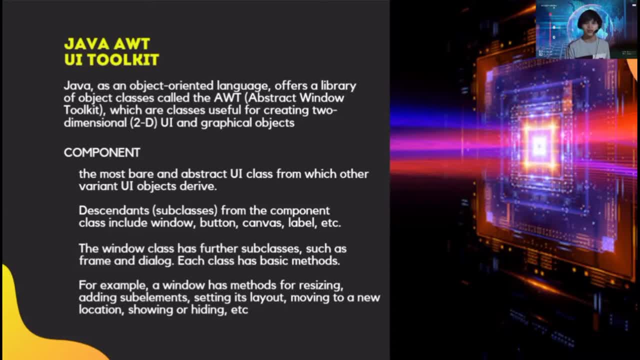 window classes for their subclasses, such as frame and dialog, and each class has basic methods. so the window class is for their subclasses, such as frame and dialogue. so, for example, a window has some methods of resizing: adding sub elements, setting its layout, moving to an indication or showing or hiding or etc. okay, so again the java java out toolkit has 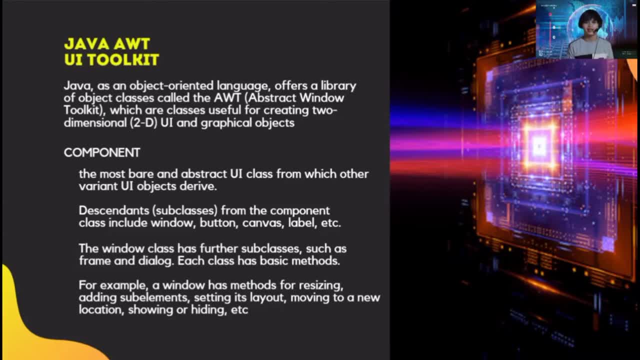 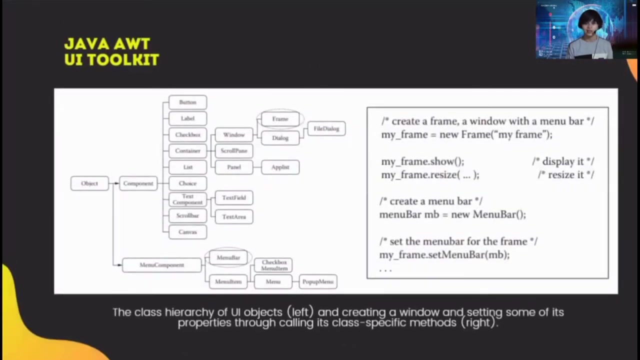 its components, okay, and then the components has different subclasses. that includes the window button, canvas, label, and a window has the control mode, has a subclasses, which are the frame and the dialog. okay, So that is the out, okay, The Java out UI toolkit. 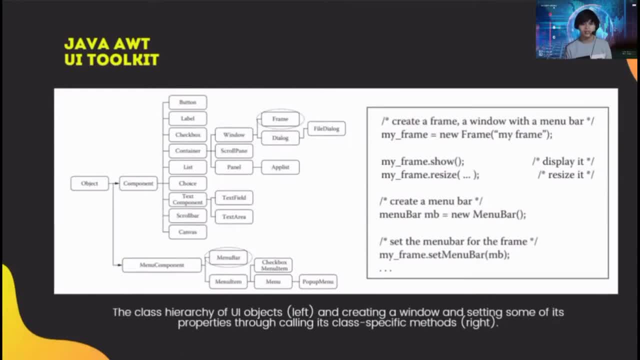 So this is the hierarchy of UI objects and this is how, actually, this is how you create it. okay, From the object there is a component and the component has different. you know. it includes button, label, checkbox, container, list choice. 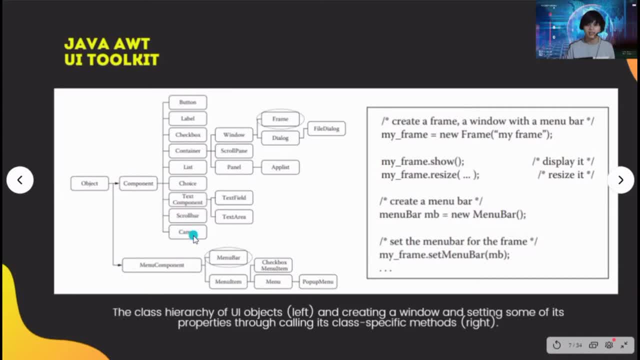 It also have text component, scroll bar and canvas- okay. So just imagine that the components has this different component, okay, And in a container it includes window scroll pane and panel. okay, And in a window it has frame dialog. 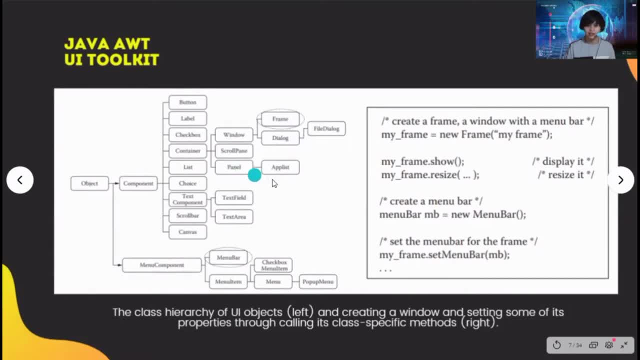 and in dialog it has file dialog okay In a panel. In a panel it has app lists. In a text component it has text field and text area okay. So imagine you design. you have this design now okay. 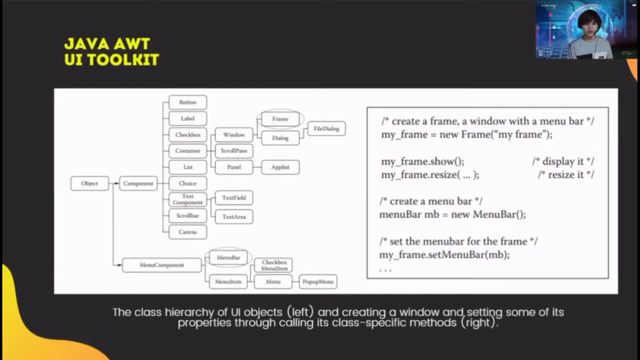 Like in page. you have this image, you have this input, you have this buttons. but ask yourself: how are you going to? you know, make it functional, okay. So in Java, there is a toolkit. okay, There is a toolkit called out. okay. 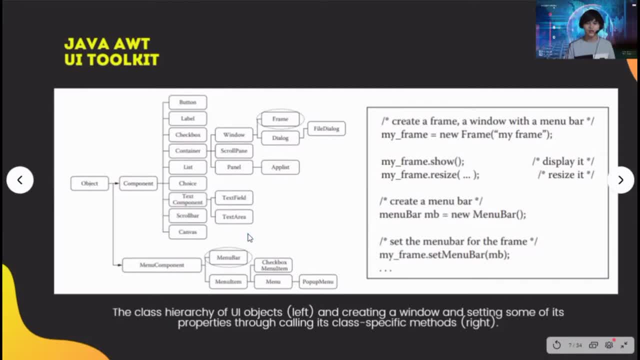 And components. okay, So in a menu component it has, of course, menu bar, menu item, checkbox, menu item menu and pop-up menu. So here's the example code for that one In here. what happened is you create a frame. 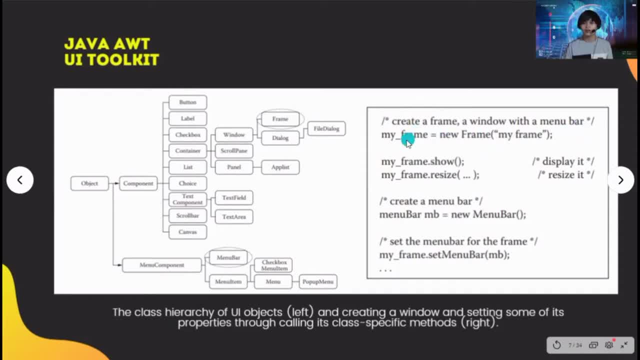 Now you create a frame, a window with a menu bar. So you have: this variable is equal to instance, right? So you create a new frame. okay, And this is the sample code. This is the Java sample code. Okay, so it would be very hard. 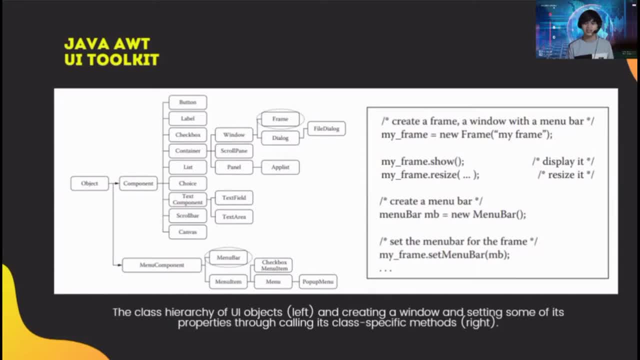 if you don't have this programming knowledge language, but this is how it is being made, okay, So just get the idea. So this one is the hierarchy of the UI objects and creating a window and setting some of its properties through calling it class, specific methods. 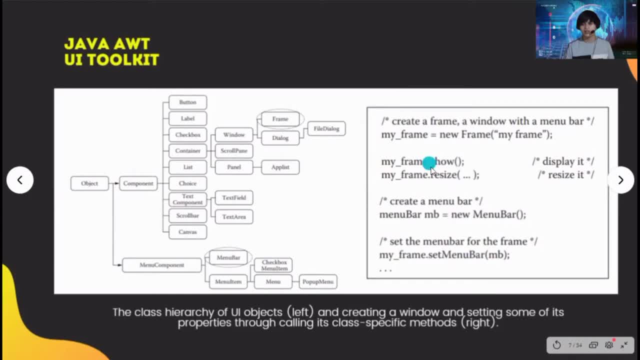 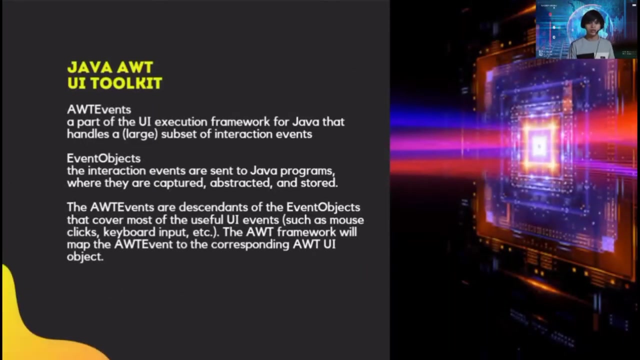 or to the right. Okay, what happened in here is this: that show method- well, can I display it? And that resize method will resize. okay, And this actually really involves methods programming knowledge kit, okay, Okay, so the Java out UI toolkits. there is also what we call 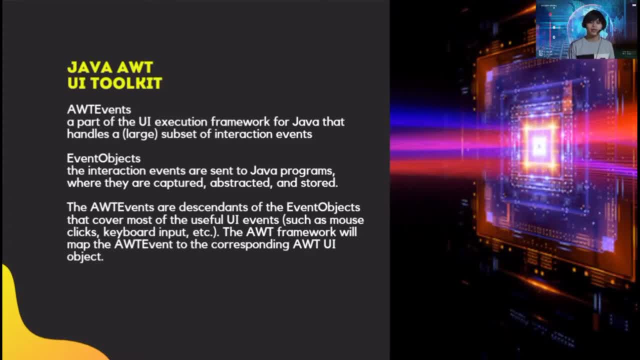 the out events. the out events. this is a part of UI execution framework for Java that handles a large subset of interaction events. okay, So in an out events there is also an event objects. This is the interaction. events are sent to Java programs. 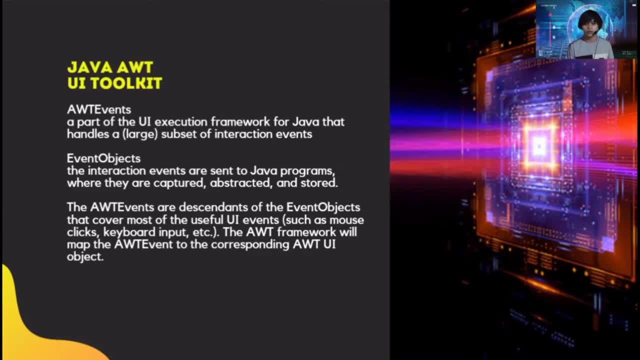 which were are captured, abstracted and stored. So the out events are descendants of the event objects that cover most of the useful UI events. that cover most of the useful UI events. that cover most of the useful UI events such as the mouse clicks, keyboard input and et cetera. 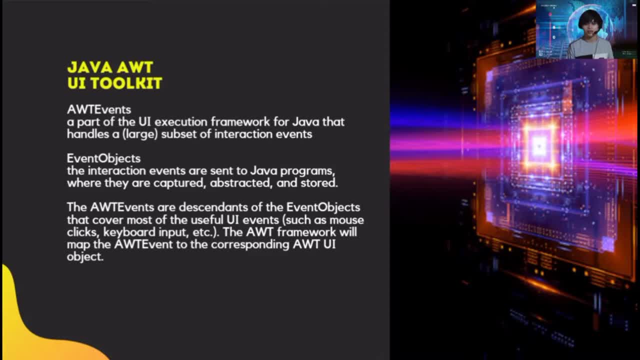 or anything resizing something like those things. The out framework will map the out event to the corresponding out UI object. okay, So again, consistency: out events. these are part of the UI execution frameworks that handles subset of interaction. The event objects are the events. 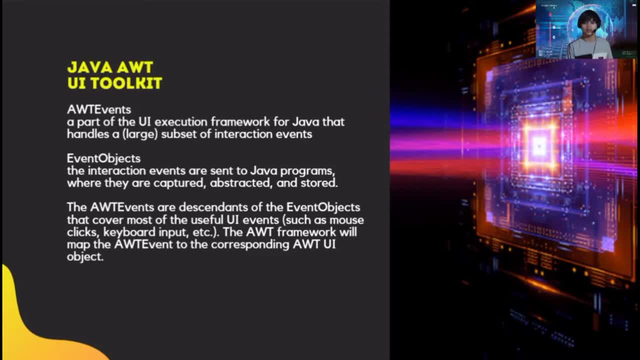 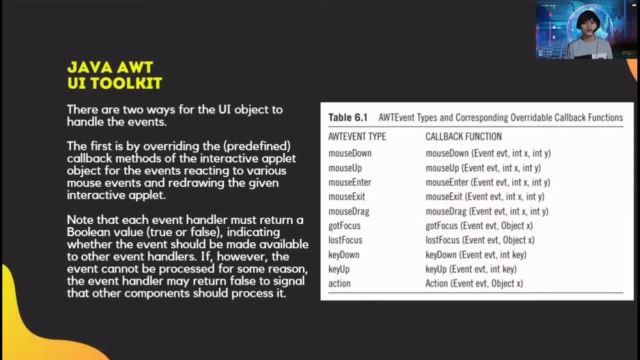 that are sent to Java programs which are captured, again abstracted and stored. okay, So there are two ways of the UI object to handle the events. The first is overriding the pre-defined callback methods of the interactive Applet object for the events. 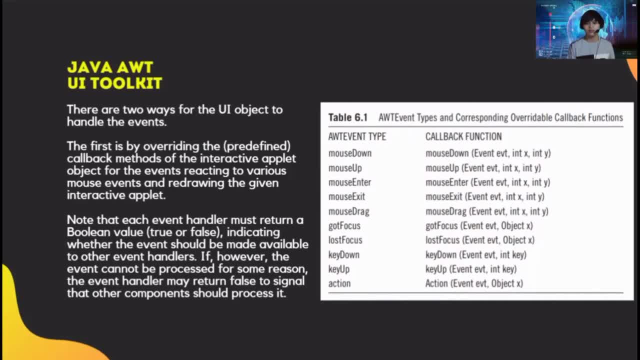 reacting to various mouse events and reviewingiver previous cost interactions. Basically, in HmM collection we are getting a set of data objects fromém redrawing the given interactive applet. so note that each event handler must return a boolean value, true or false, indicating whether the event should be made available to other event handlers. 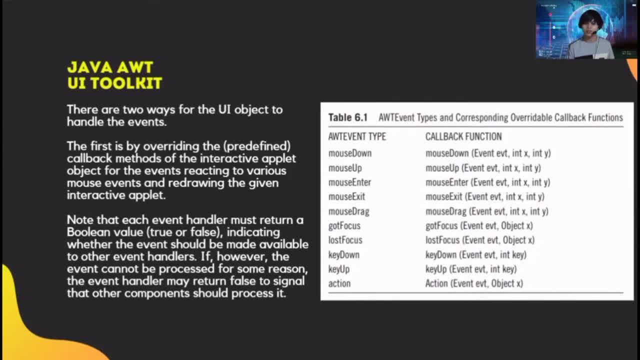 if, however, the event cannot be processed for some reason, the event handler may return false to signal that other components should process it. okay, so we have this: different event types and then the callback function. so when, when, um, when, your system has this different functions wherein mouse down, mouse up, mouse enter, mouse exit, mouse drag, get focus, last focus, k down, k up, action. 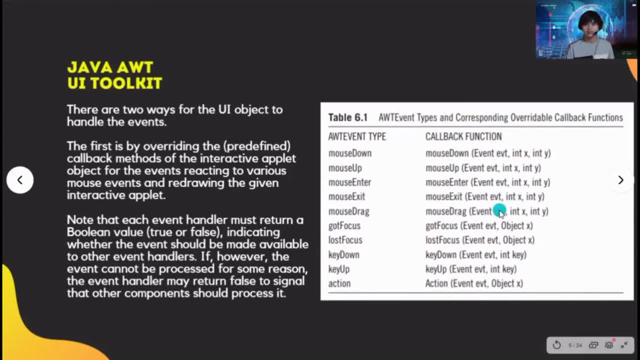 the callback function is going to be like this: okay, so again, in programming guys, you just need to include: import the library, now import the out java toolkit and after, in importing that library, you can now then use these different functions. okay, these are the different callback functions, which is you're just going to call this, you know a library, because it is, is, um, it's already. 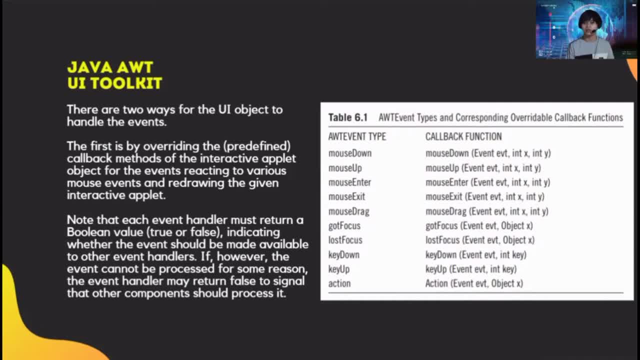 up a piece of program: we're in naana, say my different functions said: don't want to go nalang limo for you to show on an output, okay, okay. so as for the mouse down, the method, mouse down and then just put in the event, and then these are the different uh parameters. okay, and then different values. 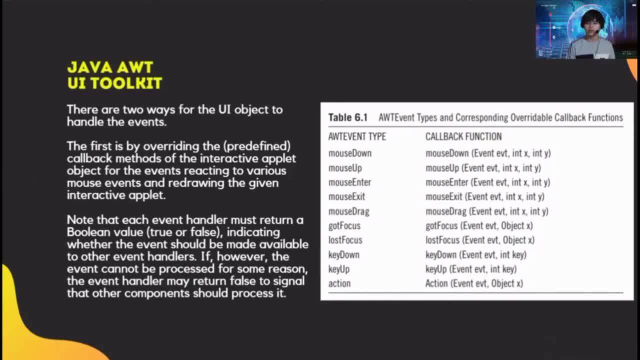 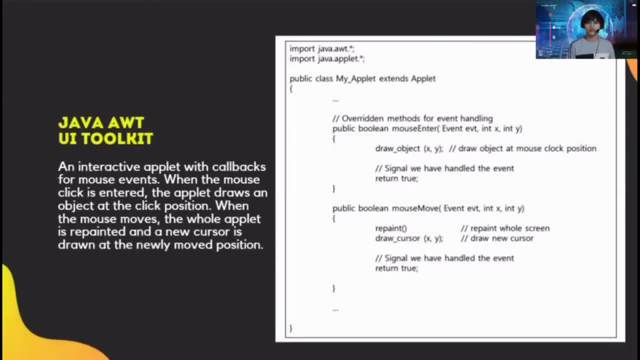 um, if mouse down scroll, yeah, if mouse click input, then this is the data for the applet. okay, so this is an example: an interactive applet with callbox for mouse events. when the mouse click is entered, the applet draws an object at the click position. 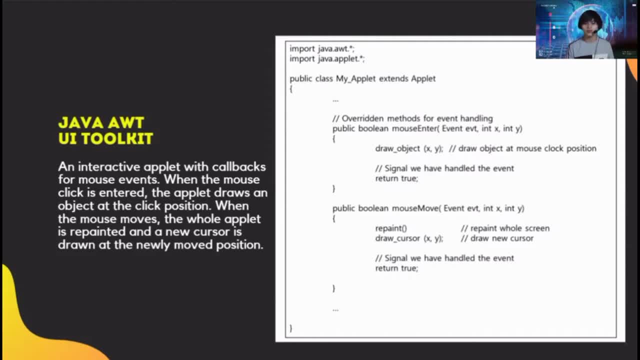 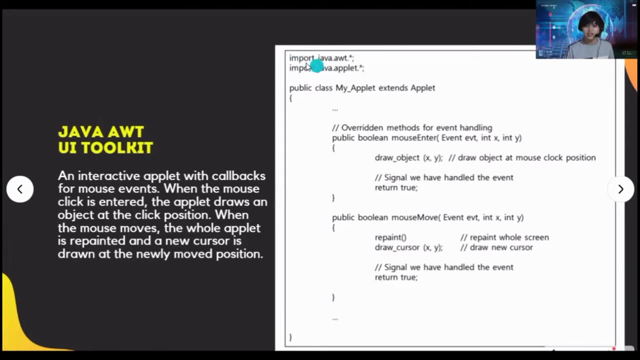 so when the mouse moves, the whole applet is repented and a new cursor is drawn at the newly moved position. so this is is this is how it gonna happens. as you can see, in our first and second line we import the java out. asterisk means all, all, uh, all libraries from the out, and we also import the java applet. so imagine: 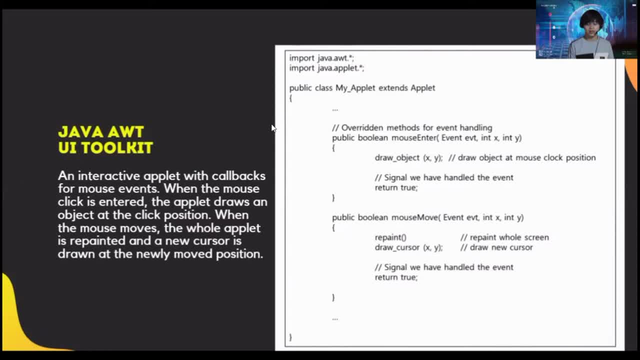 that when you have this design example, designer, and you give it to a developer, then the developer will going to create it using java code, using java programming language. so this is how it looks like. okay, just get the idea on you. get on senila, because this is another course. now input, if 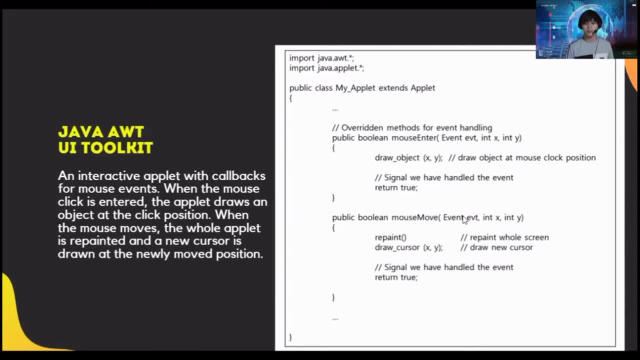 you wanted to study programming, okay, so in here just a sample. um, the developer created a public class. my applet extends the applet, now the applet library, he extends the class. so in here again, when the mouse click is entered, the applet draws an object. 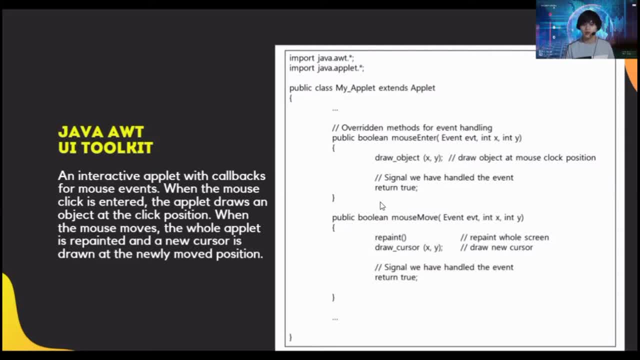 at the click position. okay, so when the mouse moves, the whole applet is repainted and any cursor is drawn to a newly moves position. okay, so this is the code, yeah, so, uh, don't worry, because we will not be discussing everything about programming, just get the idea on how the developer's going to. 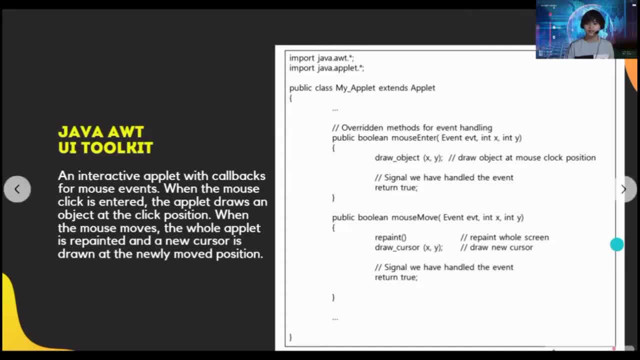 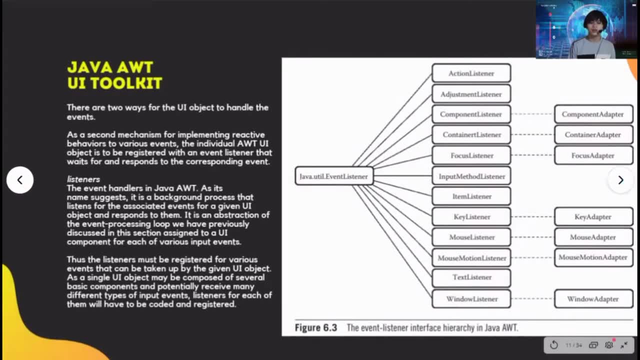 create it. okay, next, so this one. so there are two ways for the ui object. again, this is the first one. now we are in the second one. so, as a second mechanism for implementing reactive behaviors to various events, the individual out ui object is to be registered with an event listener that waits for. 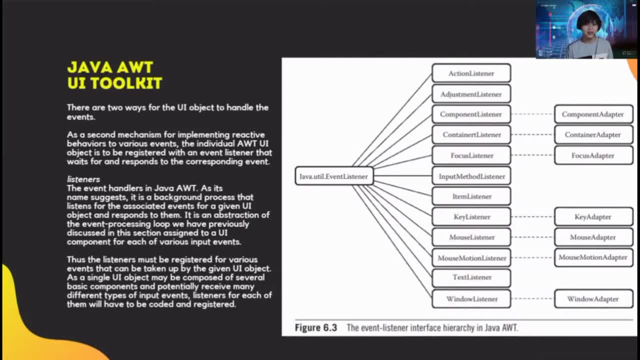 and responds to the corresponding event. now i think for me now okay, listeners. so the listeners, the event handlers in java out again, can handle some events. see listener. as its name suggests, it is a background process that listens for the associated events for a given ui object. and 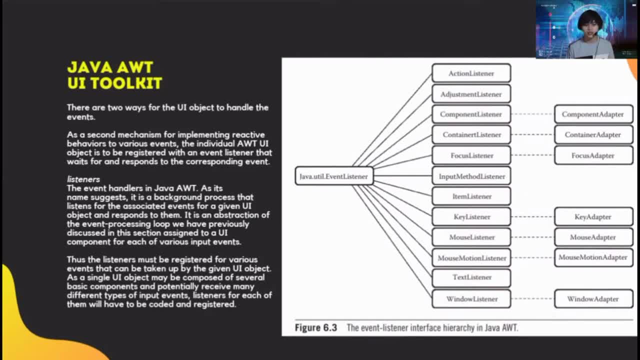 responds to them. okay, so it is an abstraction of the event processing and you have in the en απ, one or this section we have previously discussed in this section, assigned to a ui component for each of various input events. okay, i think it. it's in chapter four or chapter five. thus the listeners 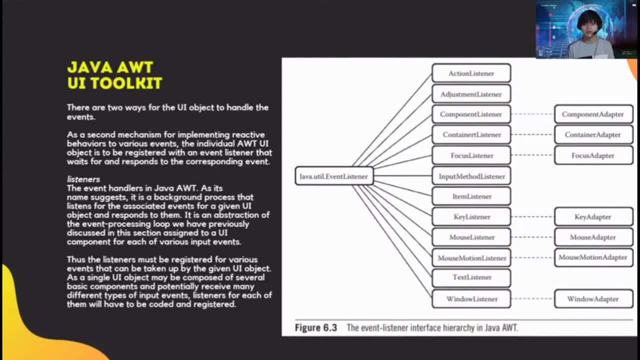 also must be registered for various events that can be taken up by the given ui object listeners, for each of them will have to be coded and registered. so again, before shama process, it should be registered to an event listener. okay, so the in java, in java out ui toolkit. 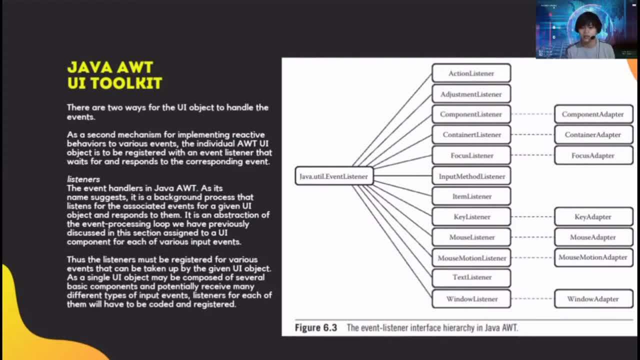 the event listener has this, has this different listeners: we have the action listener adjustment listener. we also have component listeners: container: listener focus, listener input method, listener item, listener key, listener mouse, listener mouse motion, listener text, listener window listener. so now i got a menu: say yeah, no. so again on say purpose: listener gunny, it will wait. 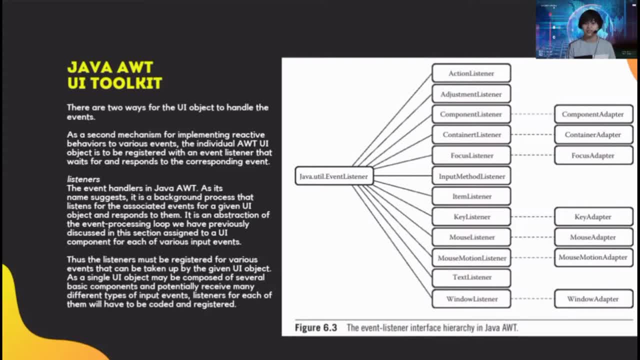 and wait for and responds to the corresponding event. okay, so uh again. but like the theory, for the component listener, it has component adapter, container container listener, it is container adapter. and in any guinness guys, um, but when in when coding, you know there are, you know, different standards, this is actually a. 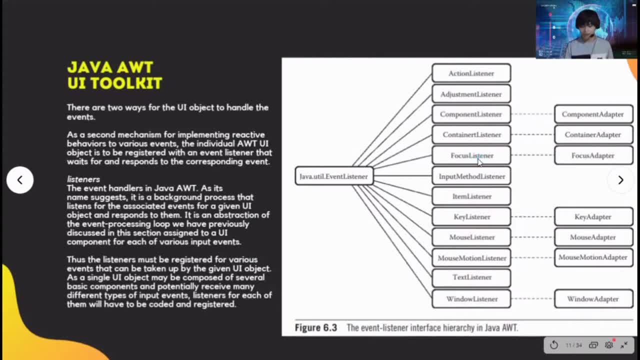 common case. yeah, i know, yeah, right, so you know again. okay, in a focus listener, it is a focus adapter. in key listener: uh, it has key adapter, mouse, adapter mouse, etc. and so on and so forth. so these are the different listeners, you know? uh, event listener interface hierarchy in java out. 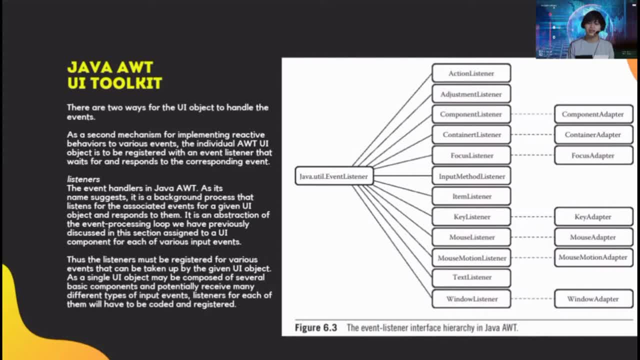 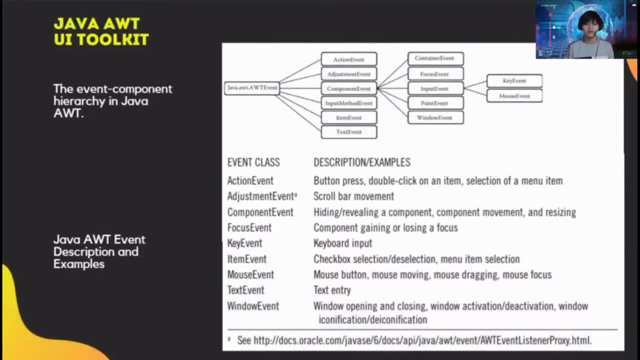 okay. so again on say purpose listener, it will wait and respond to the corresponding event game. okay, next is we have the event component hierarchy in java. okay, so an event has has action event, adjustment event, component event, input input method, event item event, text event and in the component event it has container focus, input paint. 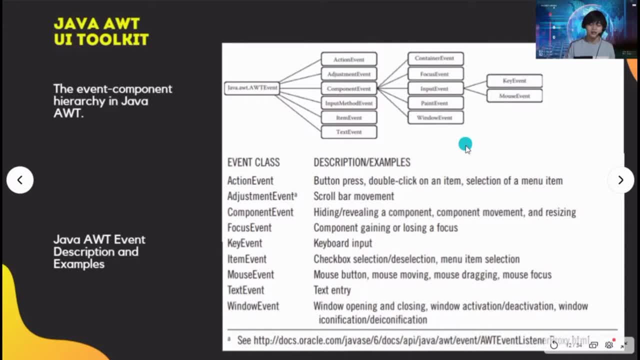 window and in an input it has key, of course, and same on input, and then the mouse event, or is it, yeah, how the mouse responds? so in action event, if the event is, if the event class is action event, the description and the samples would be, you know, button press and double click on an item or a selection of a menu item. 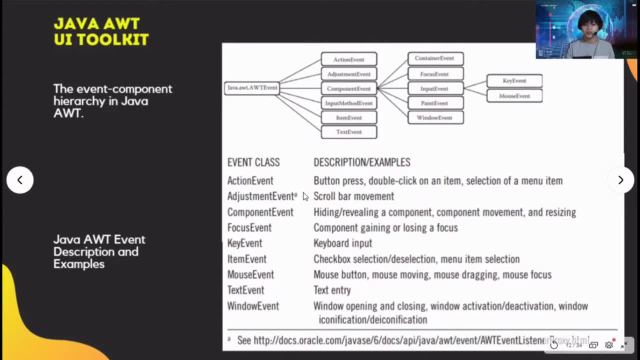 so just going to call on this function and then for the adjustment event, scroll bar movement, different type of element: read the method: electrical event. the component event is either hiding or revealing a component. component movement and resizing focus event is for the component getting or losing a focus. i think. okay, the key event is for the keyboard input. 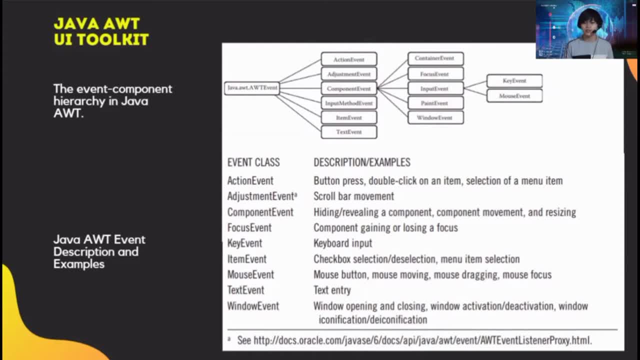 the item event is for the checkbox selection or dis-election or menu item selection. the mouse event- mouse button mouse moving text entry- and the window event is for window opening and closing, window activation or deactivation or window iconification or the iconification. okay, so again these are the different events in event components in Java out in a. 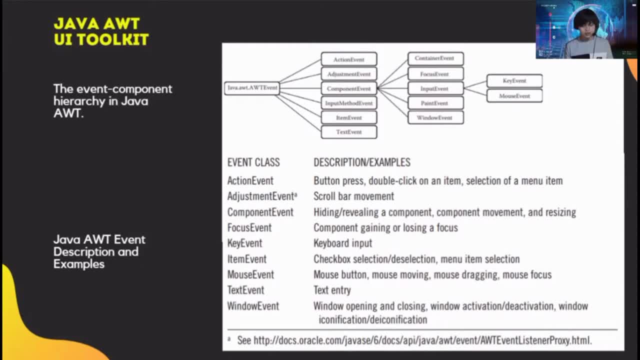 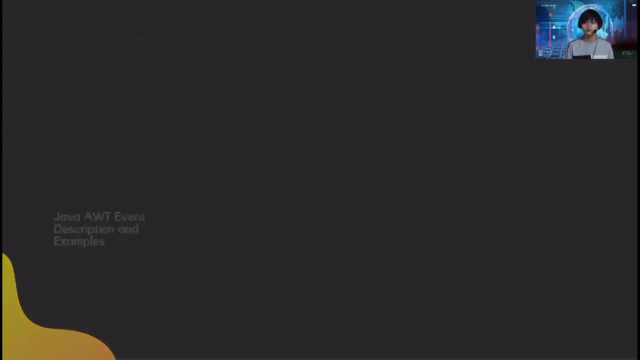 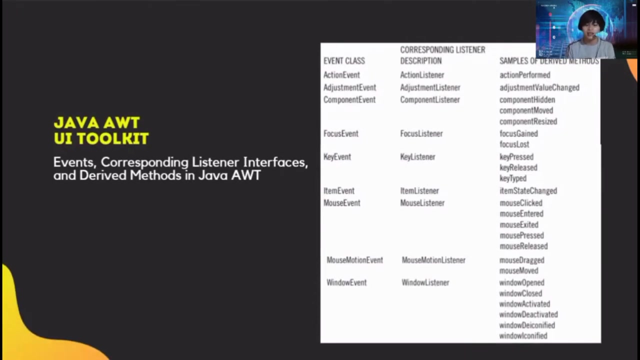 Java library, Java toolkit, rather okay. so this were the different methods. and young, young damit Kong in on sasa programmer, or you know, in society developer, but developed, okay, you know, program. so next, these are the events: corresponding listeners in their listener interfaces and derive methods in Java out okay. so let us say, for example, the event class action event. so 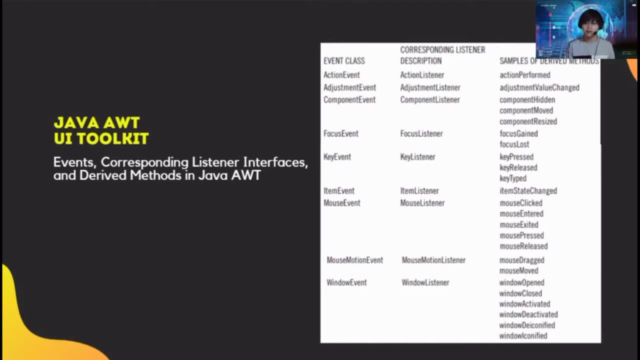 in an action event, there is again no mega Pamina. whenever event diva, there is an action list inner: okay, and for example, the method the Anna is see action performed okay. in an adjustment event, there is an adjustment listener and this sample method is an adjustment value change or so on and so forth. so these are the 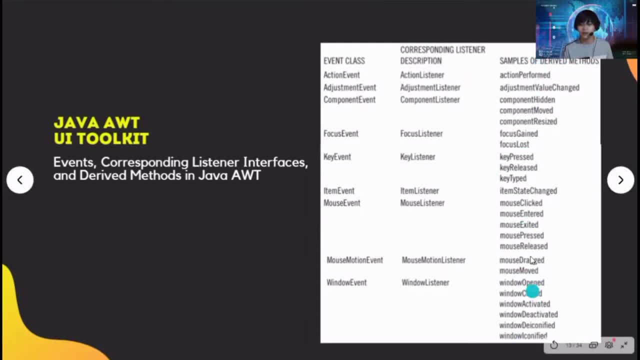 different, different derived methods. we're in the lagoon. anonymous ha Kong. it depends on the program. now. it depends on on the feature or on Sangha Sunima, my table. same on system, same on application. okay, so let us say, for example, you want the user, if, if the 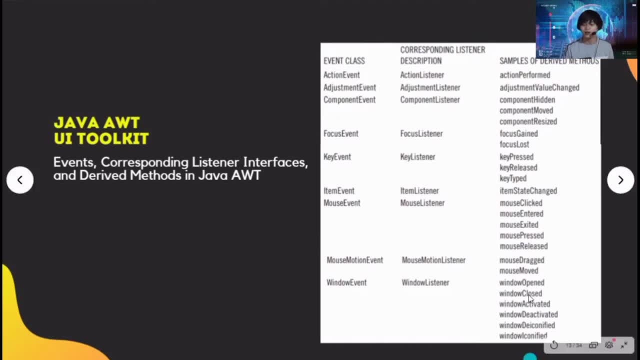 gummies of mouse. a mouse clicked? no, so once a committed method, new developer can era accessibility. mouse clicked: okay, the event is mouse event, the the description is most listener. then this are the different. there are methods. okay, so imagine, but if you have, if you have this will to develop now using this kind of language, then 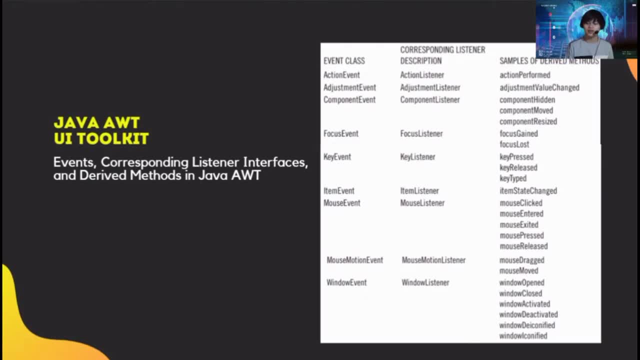 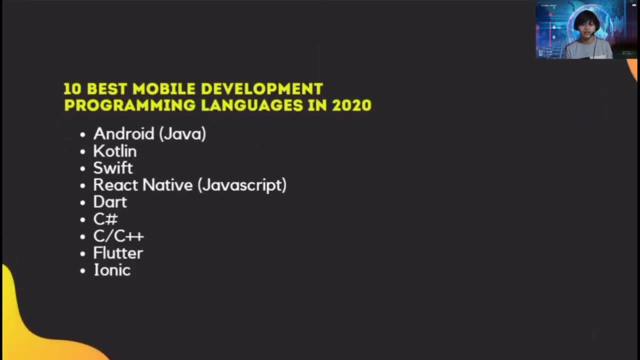 okay, so there is an event, there is a listener and there are derived methods where you can use in order for you to feature or steps on your system. okay, so next. so again, it's not only java, guys, and there are already a lot of programming languages in order for you to develop an android application or ios application or um. 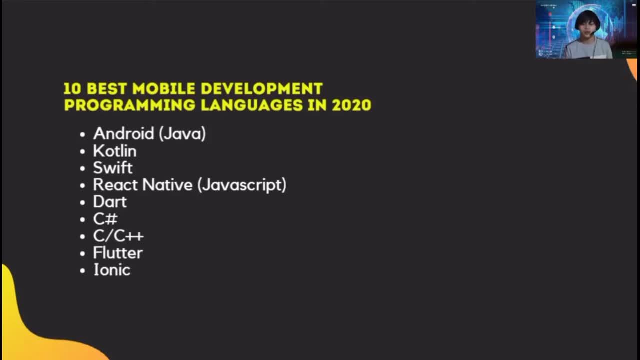 web application. so here's the top 10 as of 2020. no, we have android java. we also have kotlin, swift, react native. we have dart, c plus c or c plus plus flutter and ionic. so these are the different languages and if you want to study, so just go to their different documentations about android java. i could lean. 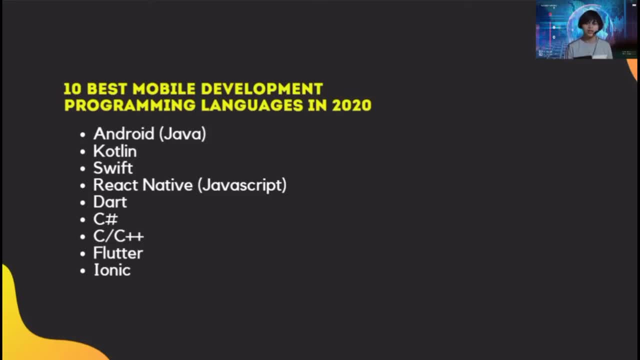 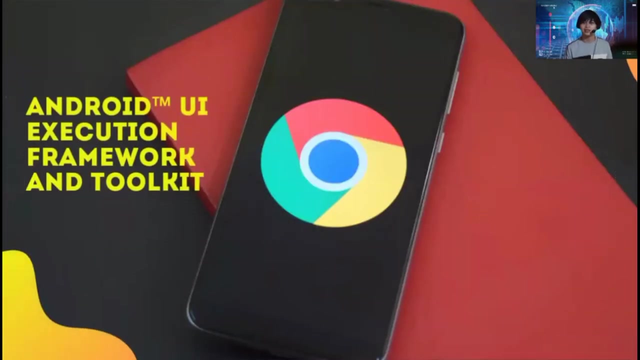 swift react native, dart c plus c, flutter ionic. there are a lot of tutorials. um, yeah, there are a lot of tutorials in the internet, so if you want to learn more, just go to their websites. okay, just go to google and search them. that's it. so that is for the java. again, what toolkit that we are going to use when we want? 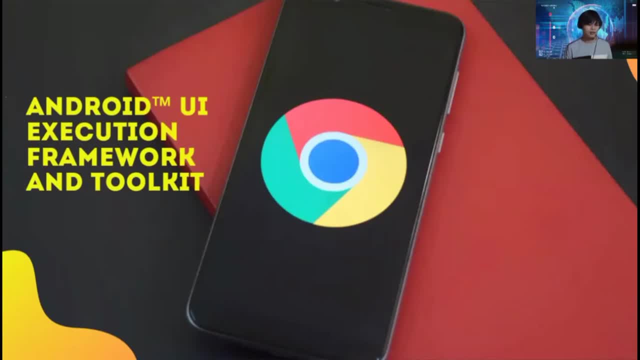 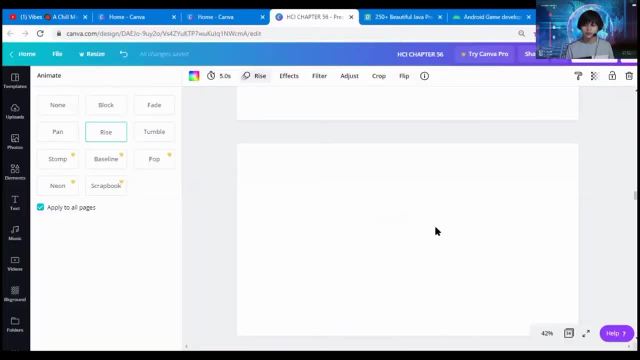 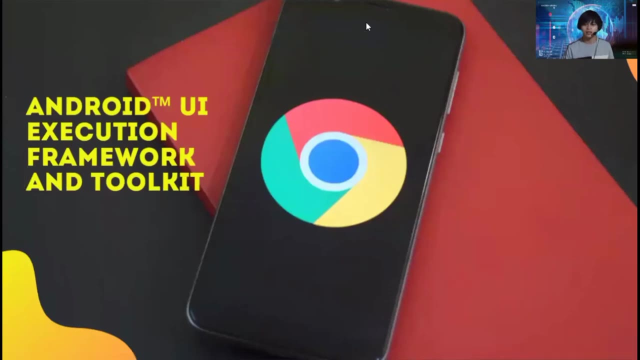 to develop a system using java. we have, they have this. you um out ui toolkit. okay, oops, wait, um, let me charge carrying again. okay, continue, not charged. so let's move forward with the android ui execution framework and toolkits, or, if you want to design an android application, and what kind of different toolkits. 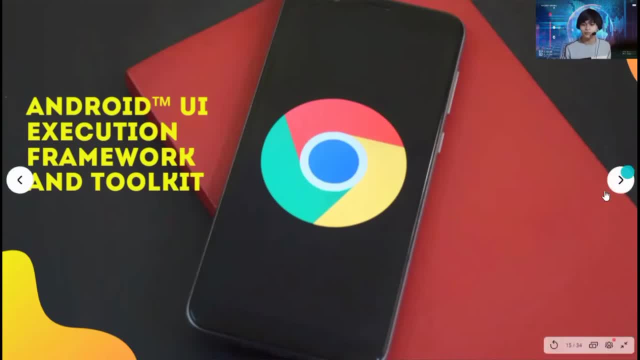 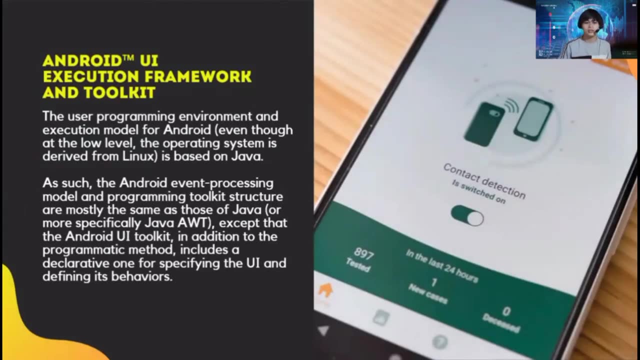 okay, knowthat, if we want an android or if we want a 56 constraint unique one, but let's just talk about the java framework. for example, if we want an going part, if we want a frontहc out, you know we, we know that, we know the java out toolkit right. so, except that the android ui toolkit, 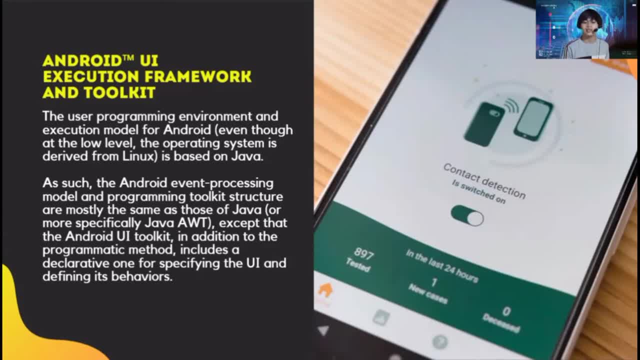 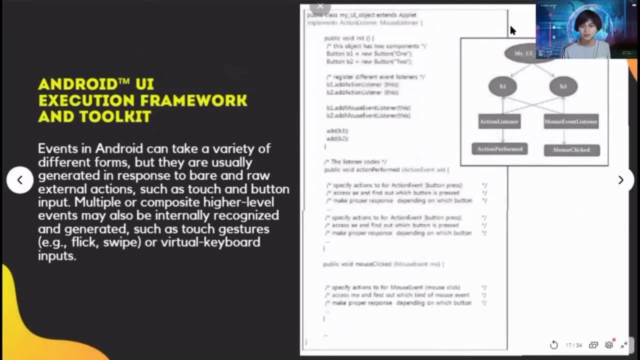 in addition to the programmatic method, includes a declarative one for specifying the ui and defining its behaviors. so for the pariah, this is android, okay, i know the java out toolkit, okay. so here's the example. i think blurry necessary new, but i'll just check the pdf, but uh. 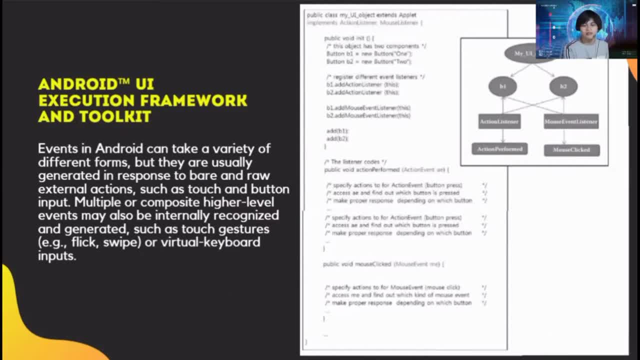 okay. so events in android can take a variety of different forms, but they are usually generated in response to bear and row external actions, such, as you know, touch and button input, multiple or composite. higher level events may also be internally recognized and generated, such as touch gestures, you know, flick, swipe or. 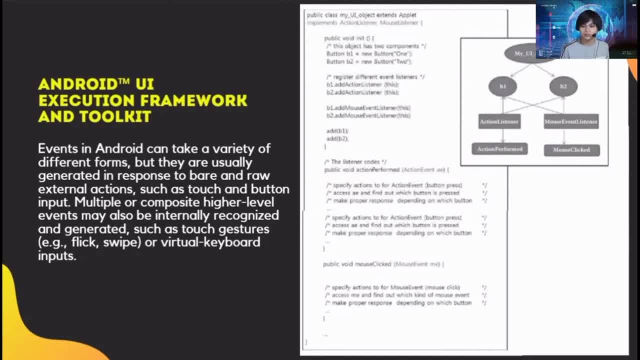 virtual keyboard inputs. so um, in here, as you can see, same same happens like error key. now this is one of the sample um and i did in a great show method: the creature, class, number, ui, object, um, again that um and content number, there is an alert. and then this one is the, the derived method. okay, so again, in an object there is always an event. 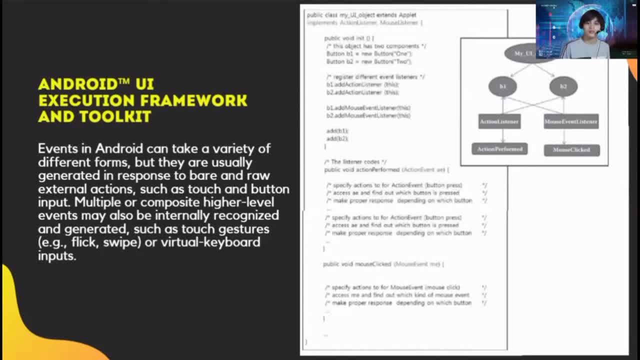 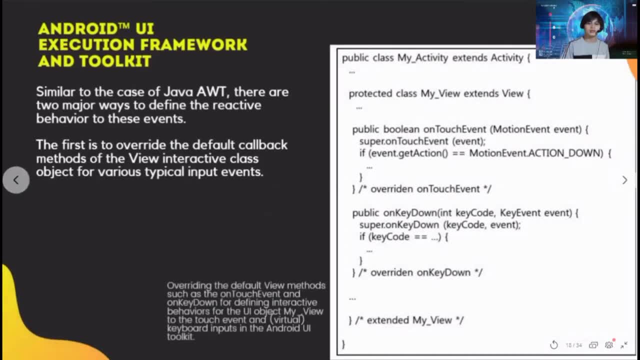 listener, and then we get the to me now, and then, um, next is the derived methods from the listener. okay, So yeah, that is the example And similar to the case of JavaOut. there are two major ways to refine the reactive major to these events. 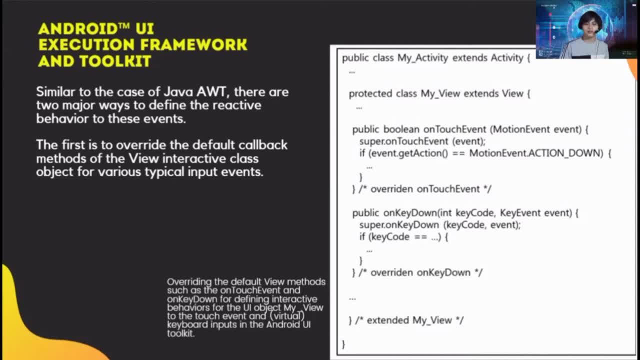 So the first is to override the default callback methods of the Vue Interactive Class. I know of the Vue Interactive Class objects for various typical input events, So this is an example. It's the overriding the default Vue methods such as the onTouchEvent and onKeyDown. onTouchEvent and then the onKeyDown for defining interactive behaviors for the UI object. 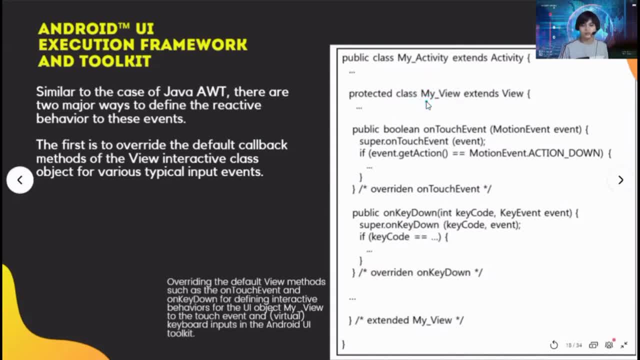 For the UI object myVue to be touch event and virtual keyboard inputs in an Android UI toolkit. So what happens actually in here is the developer created a class called myVue and then, yeah, call on the different methods, the onTouchEvent, the onKeyEvent, and then, you know, supply all the necessary parameters and 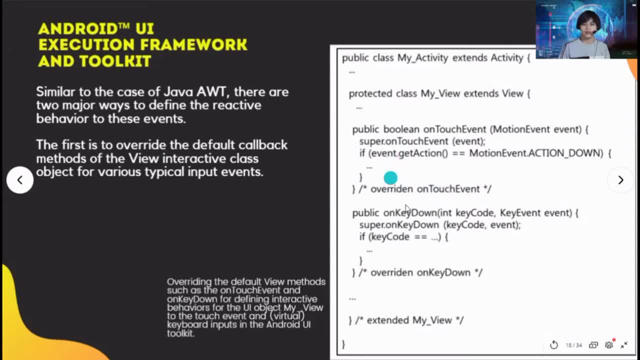 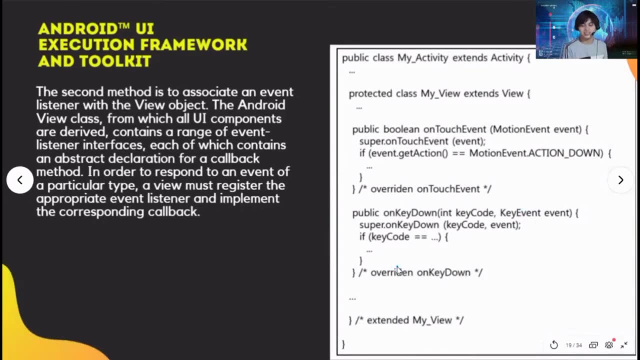 and other processes. okay, Okay, next Guys. again, it's really hard for me to actually explain it to you because it involves programming knowledge, But if you have programming knowledge it's easy for you to understand. but I hope that you get the idea of what the developer did again, what he did when he created it. okay, 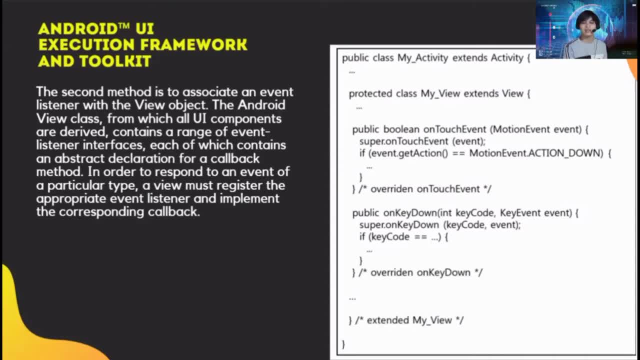 So the second method is to associate an event listener with the Vue Interactive Class. Okay, next Guys. again, it's really hard for me to actually explain it to you because it involves programming knowledge. So the second method is to associate an event listener with the Vue Interactive Class. 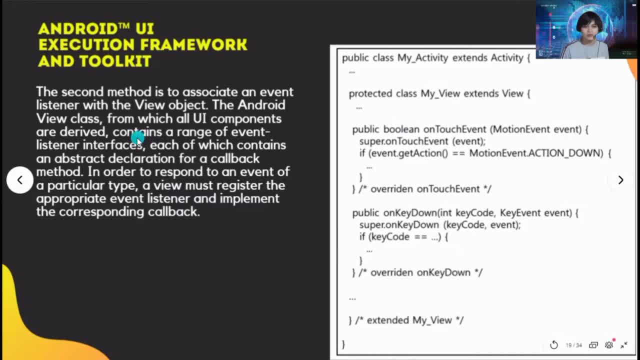 So in here, the Android Vue class, from which all UI components are derived, contains a range of event listener interfaces, So each of which contains an abstract declaration for callback method. So in order to respond to an event of particular type, a Vue must register the appropriate event listener and implement the corresponding callback. So, in order to respond to an event of particular type, a Vue must register the appropriate event listener and implement the corresponding callback. So, in order to respond to an event of particular type, a Vue must register the appropriate event listener and implement the corresponding callback. 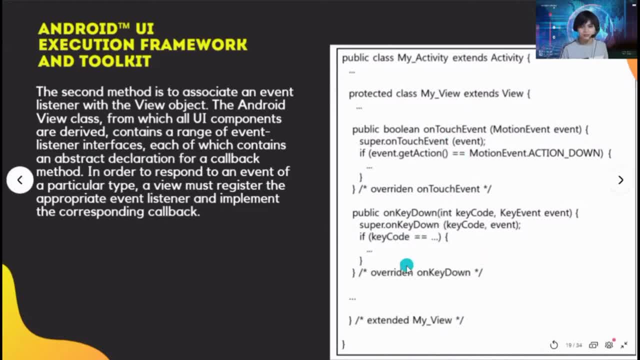 So hearts. thanks for listening. So first example: okay, Yeah, So again the Android in here. the Android Vue class, from which all UI components are derived, contains the range of event listener interfaces- Okay, And each of which contains an abstract declaration of callback method. 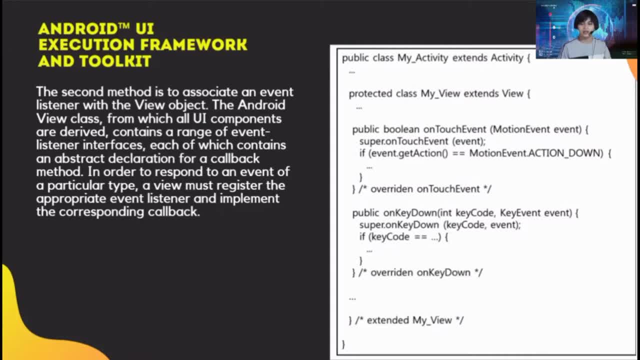 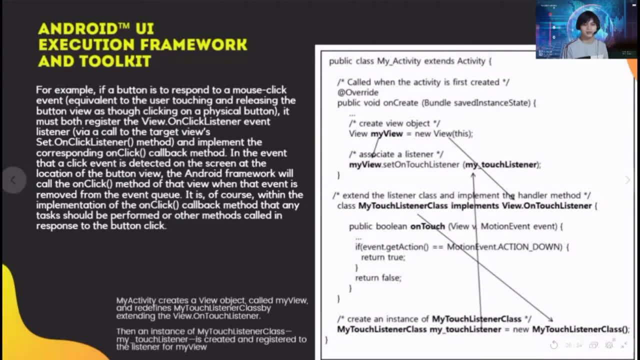 So you can call these methods and then choose which one you want to see in your application. Actually, the methods are predefined, Okay. so, for example, if a button is to respond to a mouse click event, equivalent to the user touching and releasing the button view as though clicking in. 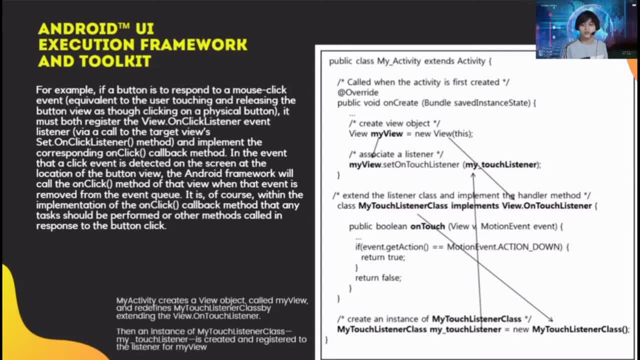 a physical button. it must both be registered to the view. Okay, so you can see in here. It must be registered the view that on click listener, via a call to the target views, set that on click listener method and implement the corresponding on click callback. 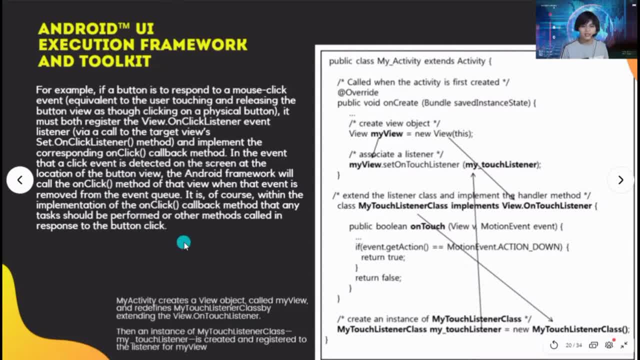 method. So in the event that the click event is detected on the screen at the location of the button view, the android framework will call the onclick method of that view when the event is removed from the event queue. so it is of course within the implementation of the onclick callback. 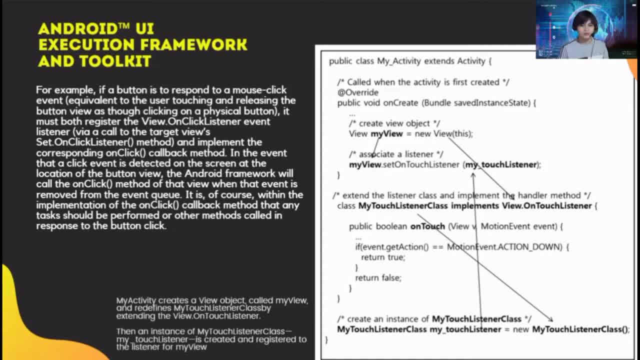 method that any of the tasks should be performed, or other methods called in response to the button click: okay. so again, um, i'm gonna try to create a class. okay, instantiate. and then canina didn't get the wog. no method, no variable monitoring. get the wog: different listener, okay. so i hope. 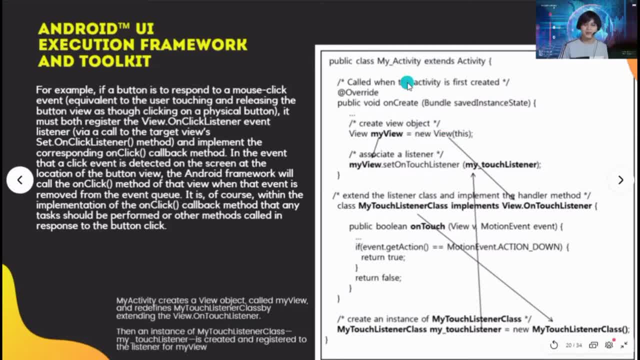 yeah, so what happens in here is that the my activity in class created a view object okay, creates a view object called my view okay and redefines my touch listener class by extending the view that on touch listener okay in here. so then an instance of my touch listener here, um my touch listener, is created. 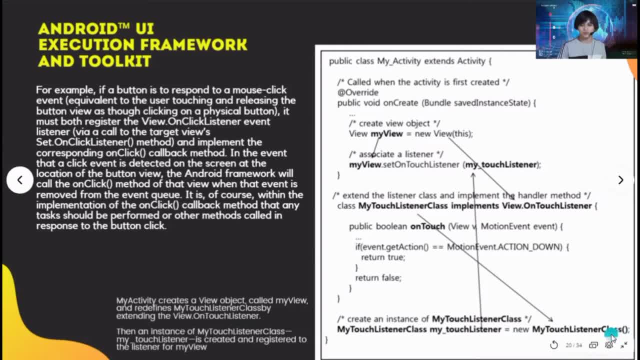 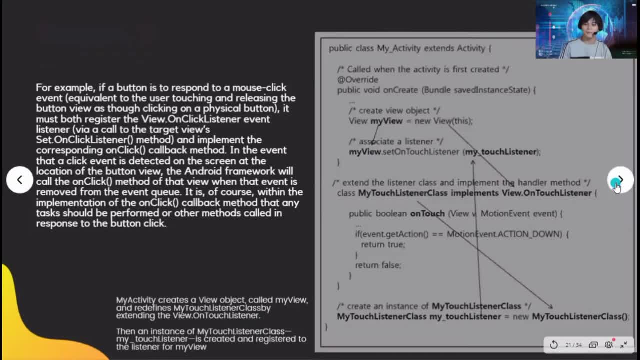 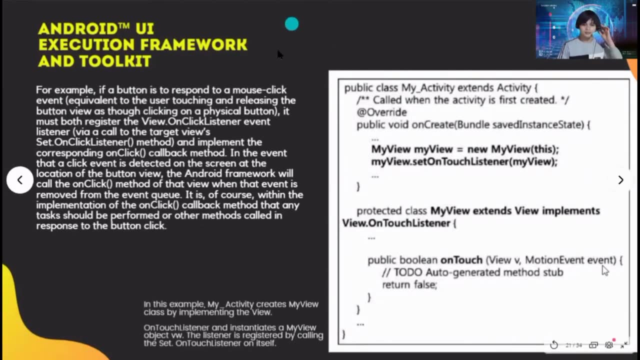 and registered to listener to my view. okay, so just get the idea: wait, wait, megane gonna pause before connect before. okay, so in this example, my activity creates my view class implementing the view. okay, and then on touch listener and instantiate a my view object: view w. okay, the listener is registered by calling the set. 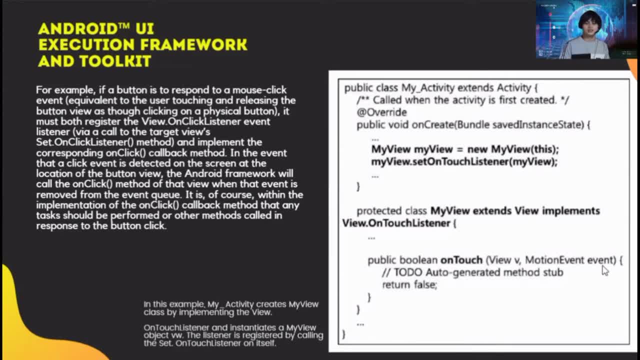 on touch listener on itself. okay. so again, it involves programming knowledge, and then we will not be discussing about the logic and the bug, but we will be talking about that later. okay, so, esta, okay. so here we go, discussing about the logic and about about the backbone and and any programming i know. 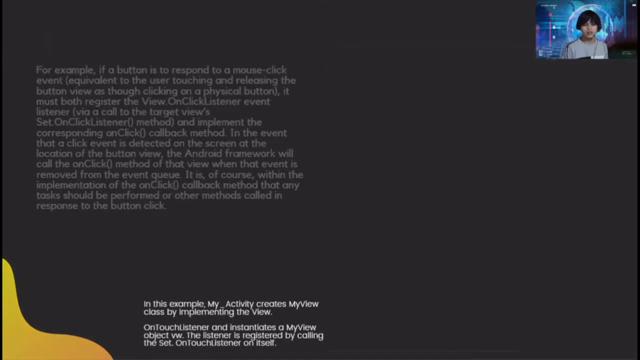 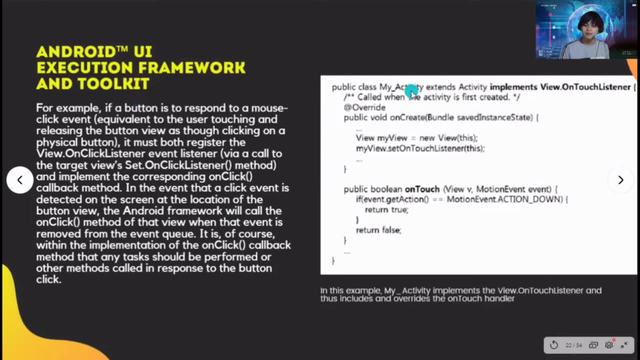 okay, it's a different course, so just get the idea. so in here, what happens in here is the my activity implements the view. touch on listener. so again, these are the different callback methods. you know library and then just call it okay and this includes an overrides on touch handler. this one is the example. okay, so it implements the view. 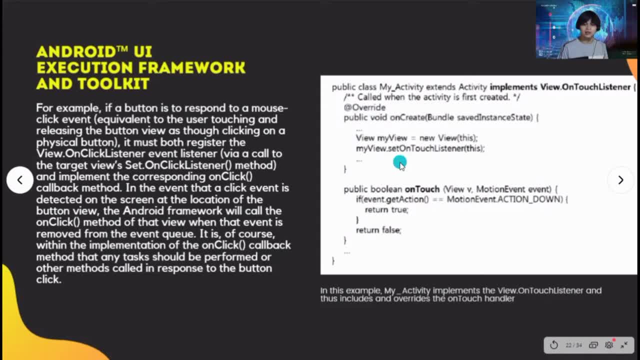 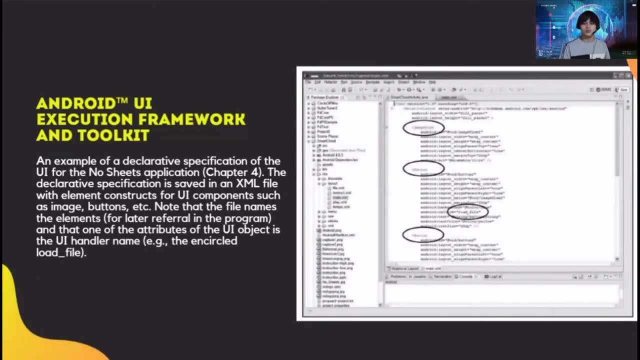 that on this listener, it override and then it creates the on touch um on the handler. yeah, so that's it. it's one of the example, okay, so again, as mentioned, uh, same, same, which is a java out, right, but then in an android it has a declarative specification for ui of the ui. 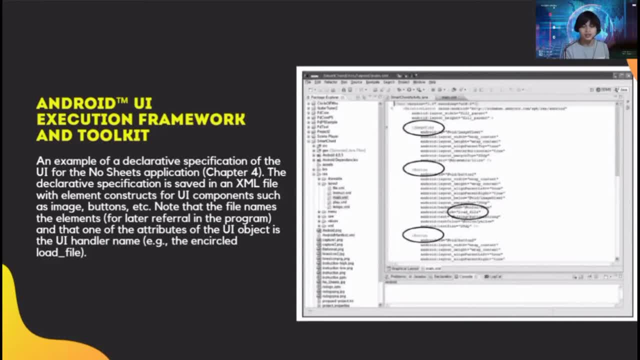 so, um, this one is the example for the new sheets application from the chapter 4. so the declarative specification is saved in an xml file with element constraint, and then it's a declarative specification for the xml file with element constraint, and then it's a declarative specification for the xml file with element. 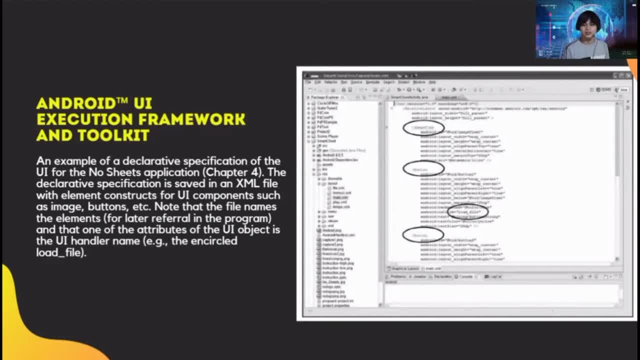 constraint. and then it's a declarative specification for the xml file with element for ui components such as image buttons- actually image buttons- and other, etc. we have different inputs, so note that the file names the elements for lateral referral on the program and the one of the attributes of the ui object is the ui handler name or the encircled load file. okay, so 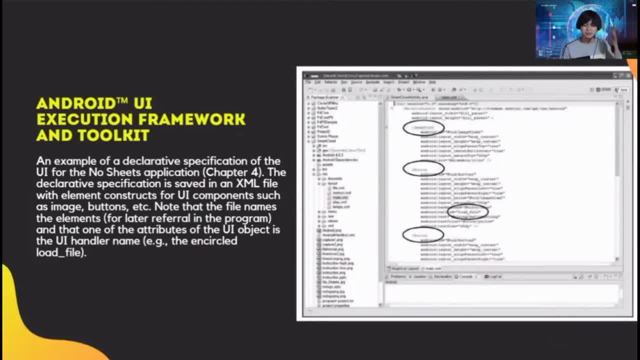 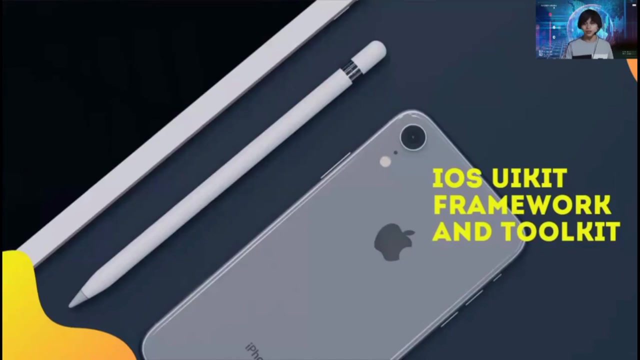 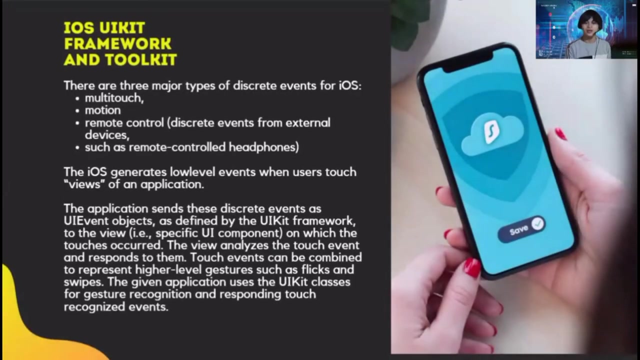 yen, it's actually really hard for me to explain everything to you guys, but killing, programming knowledge, okay. so that is how the android application works. so i hope now you got the basic idea. now let's gonna move on with the ios ui kit framework and toolkit. so in an ios there is a different three types of discrete events. 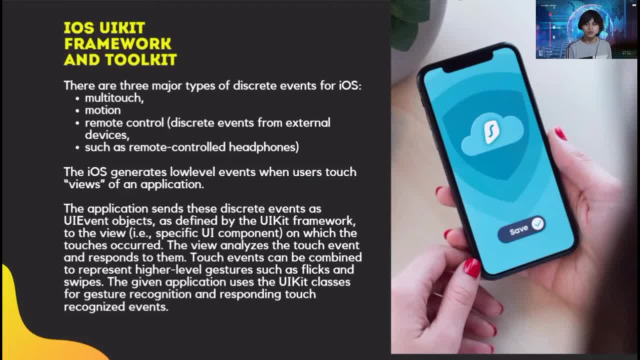 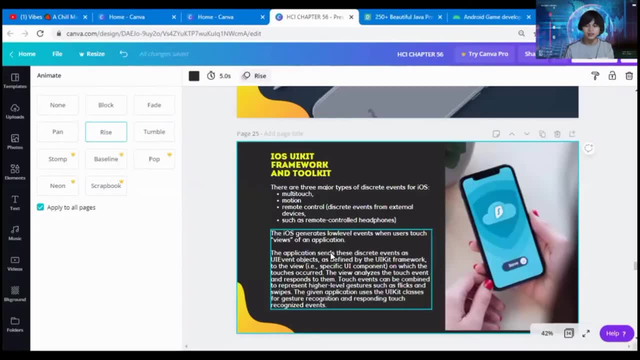 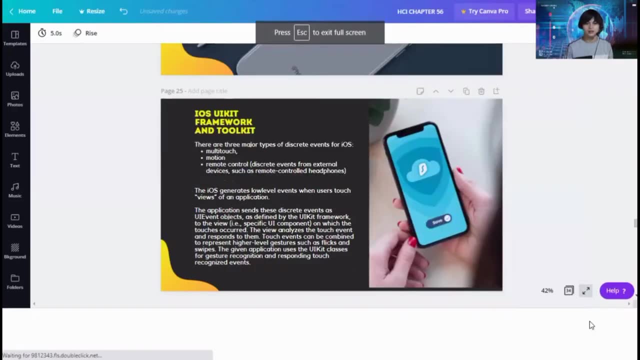 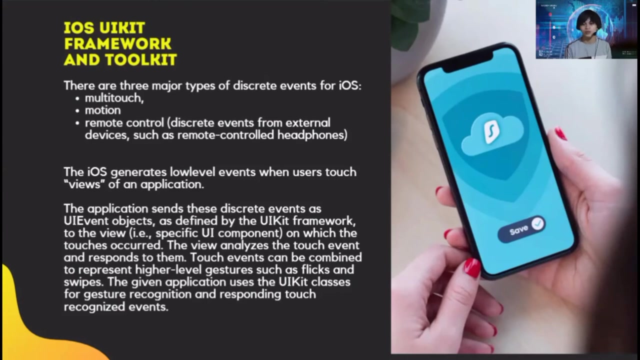 we have multi-touch motion remote control and then, yeah, remote control, wait, it should be in here. okay. so remote control or discrete events from external device devices such as remote control headphones? okay. so the ios generates low level events when users touch or views of an application and the application sends this discrete events as ui event objects. so again same pinacona when 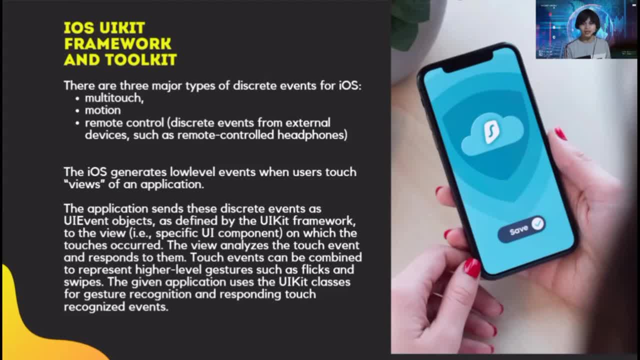 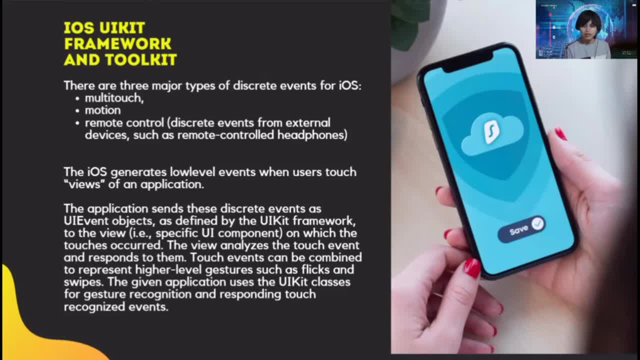 ui different components in on an ios so on which that the touches acquired the view analyzes the touch event and responds to them very often. because some users put touch frequently or if they're not familiar with touch ios outside of technical science, some users have to calculate which is the touch action using different 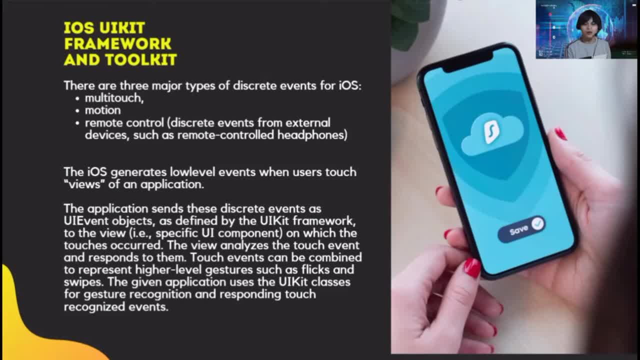 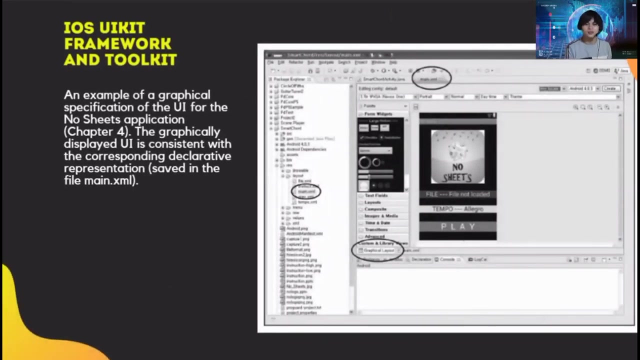 such strange learning time having different video rabbits. the touch events can be combined to to represent higher lever gestures, such as flicks in swipes. the given application uses the UI kit classes for gesture recognition and responding touch recognize events. okay, so that's it. so this one is the example of the graphical specification of the UI for the new. 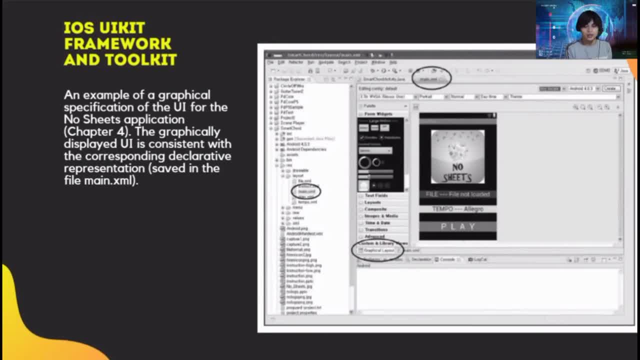 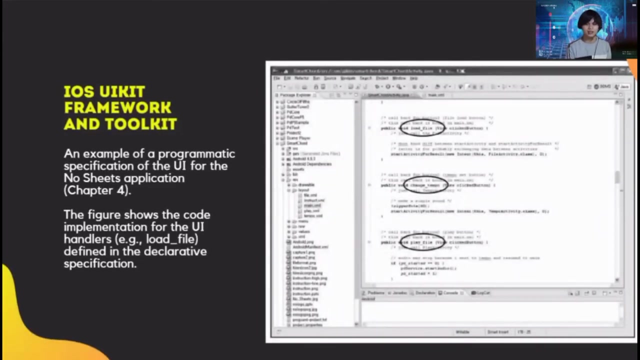 such application don't sample not. oh, it's a chapter 4, so the graphically displayed UI is consistent with the corresponding declarative representation saved in the file main, that XML. so actually this is the developer side. so not really I know. explain: begin a ton and under a month. okay, so this is the 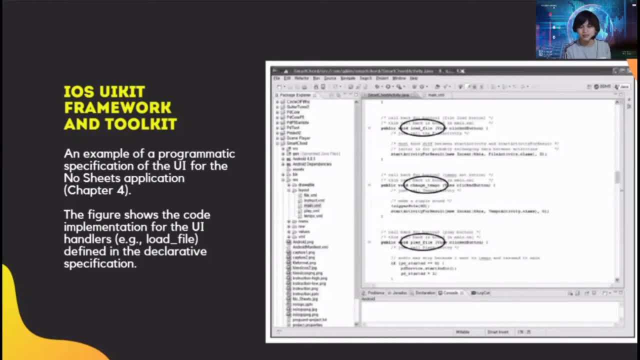 example of a programmatic specification of the UI for the new search application. so it shows the code for the implementation of the UI handlers. again the- it's the load file and this defined in a declarative specification. when you actually have this programming language, must that must easier and emotion was have done okay, so 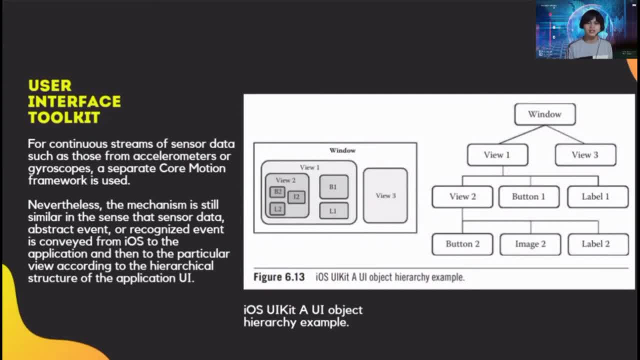 this one. for continuous streams of sensor data, such as those of the accelero, accelerometer or gyroscopes, a separate core motion framework is used. nevertheless, the mechanism is still similar in the sense that sensor data or abstract event or a recognized event is conveyed from ios to the up. 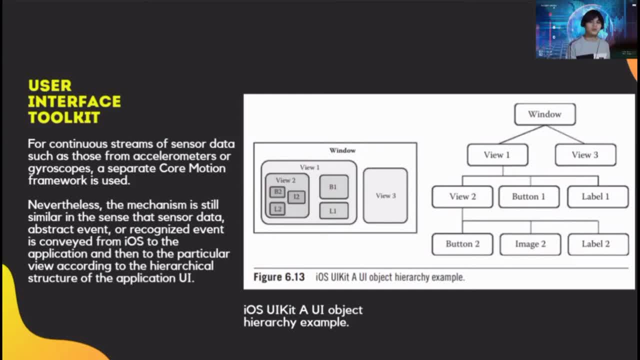 and then to the particular view. according to the aerical structure of the application, you Tell Match in a はい. so this is an example of an ios tool kit: iu, io. So this is an example of an ios tool kit- io- IO code. this is an example of an ios toolkit. you know ios. this isatha with context. this is glant management on eはい. this is also the advance communication module. a mea and dash for a architects star. thank you very much to dinner by dyed gold for computer data. you think today I will need to explain more about ağ nè the的是y. so the SEO from an actual particularparticulate- the islands- is explained all right. so this is an example of혔 as an iOS toolkitG nach Cobalt. 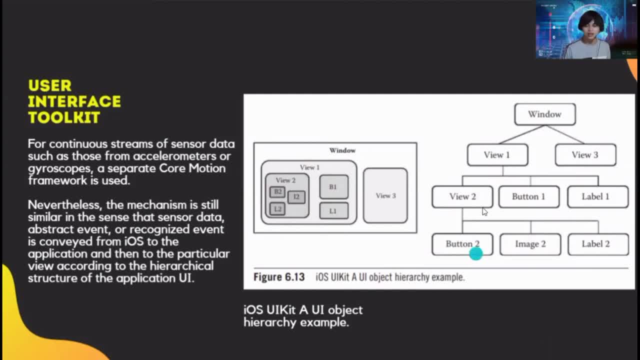 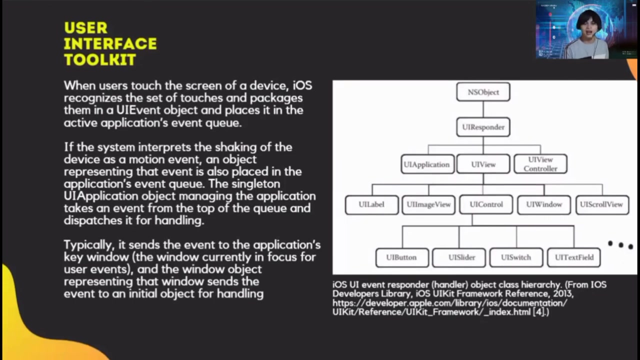 UI kit, a UI object hierarchy. okay, so there is a window, sample window, there's a view, there's another view and there's a button of that view. okay, yeah, money example. so next, so when users touch the screens of a device, iOS recognizes the set of touches in packages and packages them in a UI. 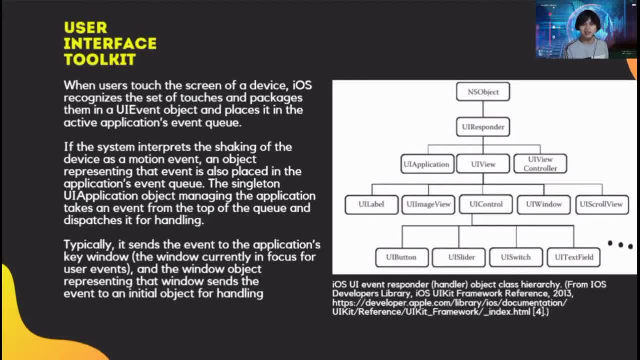 event and places it in the active application event queue. okay, and after that, if the system enter, pray interprets this shaking of the device is a motion event. an object representing that event is also placed in the applications event queue. okay, so the singleton UI application object managing the 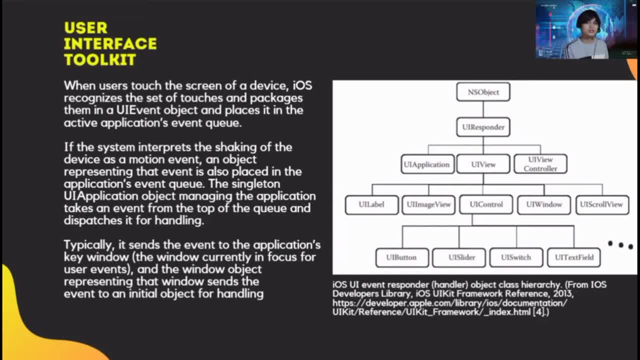 application takes an event from the top of the queue and then dispatch it for handling. typically it sends the event to the applications key window, the window currently in focus for user events, and the window object representing that window sends the event to an initial object for handling. okay, so that is how. 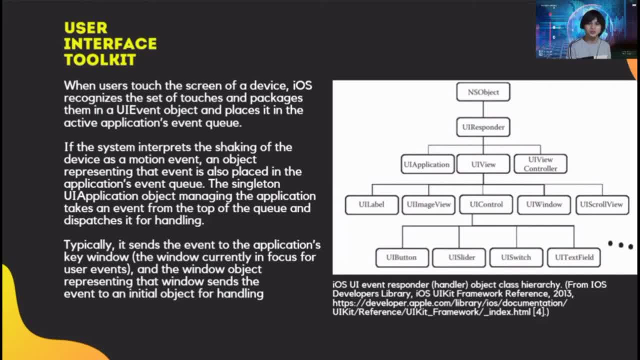 it can happens, if what I can emotion, as I've done, then go back to in here, basara, so again, with the user sets the screen neighboring eyes, iOS recognizes the set of touches. so you imagine, okay, imagine not only more, in fact, and packages any patchage into UI event and after. 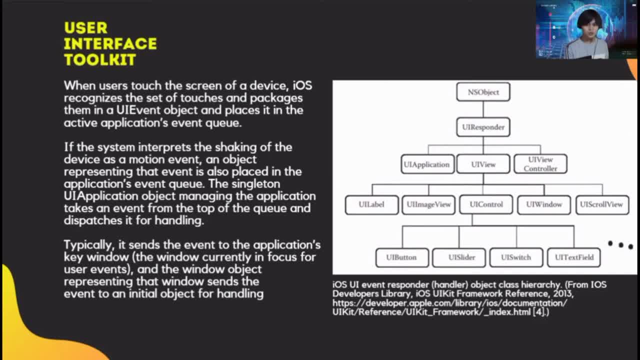 that it places in an active application event queue. okay, then look at this money and your Kacon article. say yeah, yeah, so simple as that. so they'd like an from reallyori the new chat. okay, there is just always wiggle room, just like that. please, to show up in a few times. I'm trying to begin with, so there's a besides. I just like just pass. 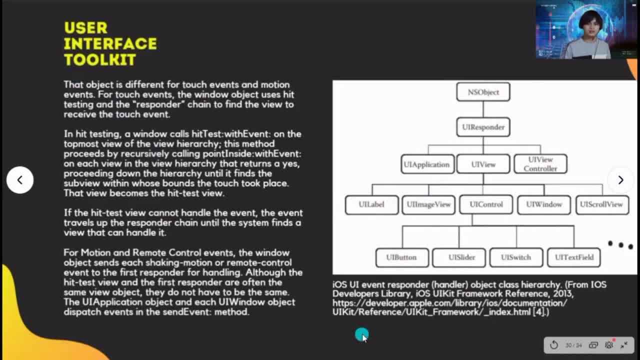 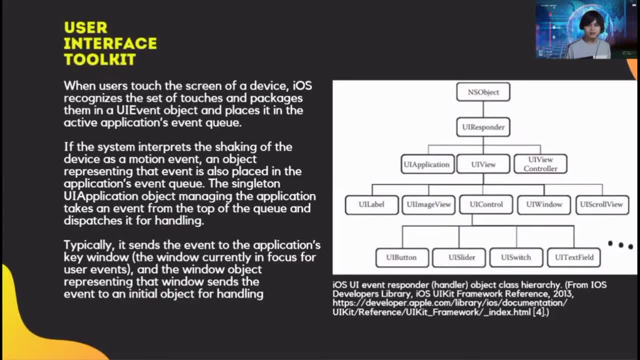 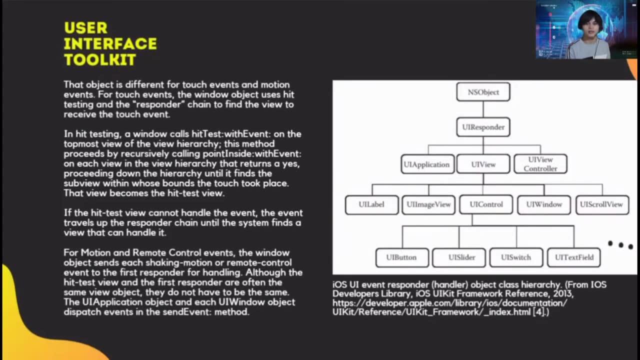 is struggle for you to discuss. okay, continue, oops, continue. that object is different for touch events and motion events. so for touch events the window object uses hit testing. okay, so touch event to window object: the use of hit testing and the responder chain to find the view to receive the touch event. so in hit this thing a window, 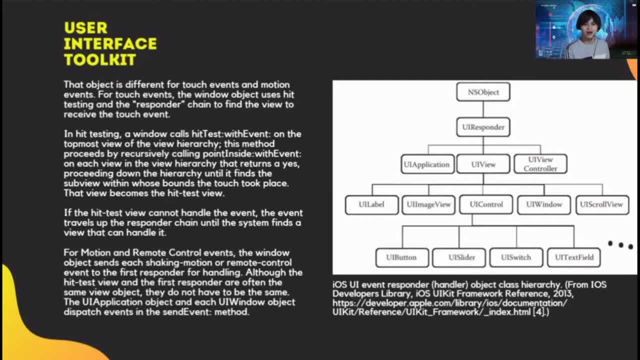 calls hit tests with events on the topmost view of the view error key. so this methods proceeds by recursively calling point inside with event on each view in the view hierarchy that returns a yes, so proceeding down the hierarchy until it finds the sub view within those bounds. 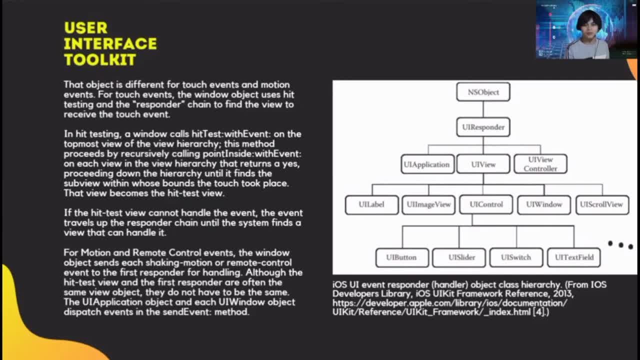 the touch took place, so the view becomes the hit test view. so if the hit test view cannot handle the event, the event travels up to the responder responder chain until the system finds a view that can handle it. okay, so for motion and remote control events, the window object sends its um. 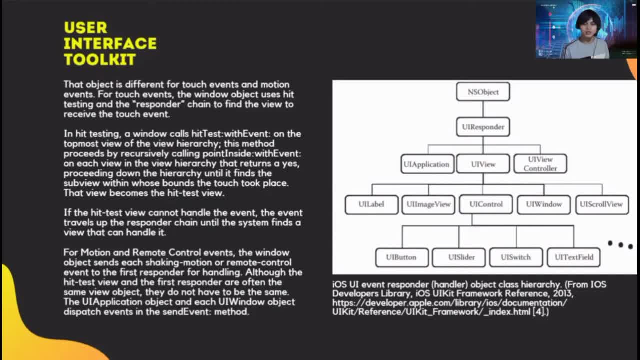 shaking motion or remote control control event to the first responder for handling. although the hit test view and the first responder are often are often the same view object, they do not have to be the same. so the ui application object and each ui window object dispatch events in the same event methods. so again, guys, 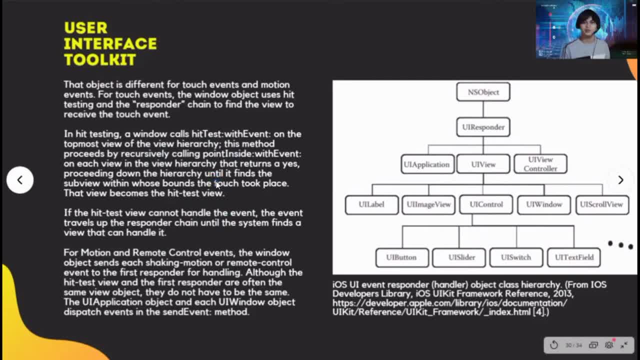 another is a different methods, when, when we call on the those different events, okay, when now, i guess, so now can i am a hitable, same system. so again, um, it involves programming knowledge, but this is the hierarchy, this is sample hierarchy, this is the event, responder, object, class hierarchy. so in an object there is a responder and from that responder. 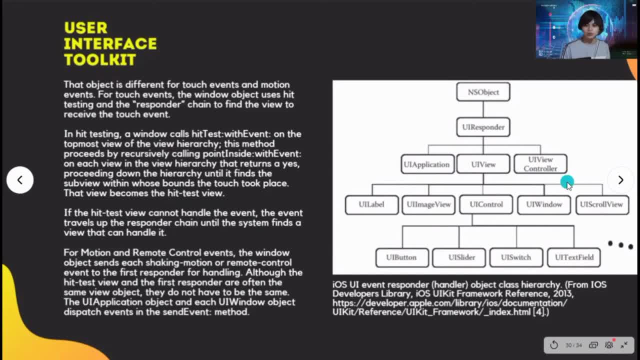 there are applications: ui view, ui view controller and then for the ui view there are, you know, when you want to display level image view, ui control window, scroll view and in a ui control there is button slider, ui switch, ui text field. so actually, if you have this programming knowledge and 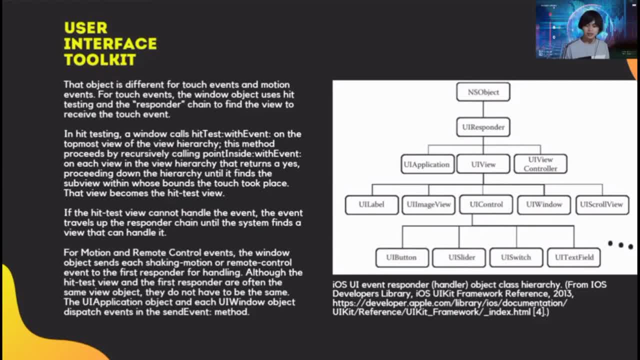 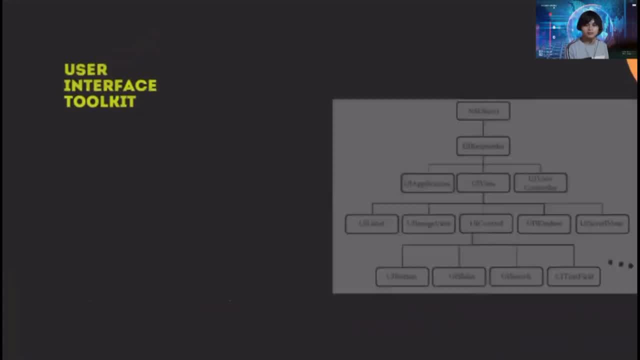 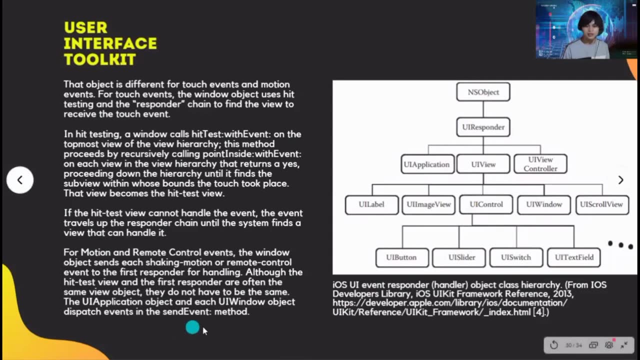 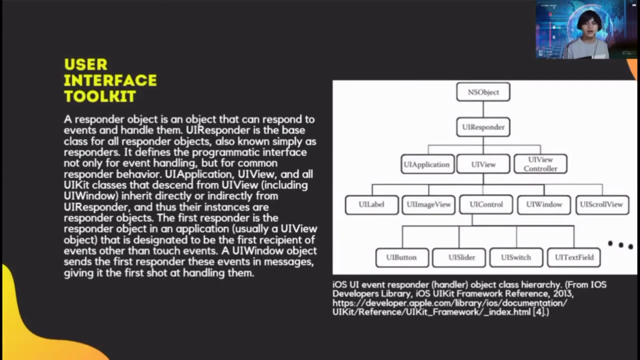 programming skills. it would be easier for you to understand this. and mustalita, same one. yeah, dokum, look, you are over here. thanks, thank you one more time, my old eyes. what is this? So it defines the programmatic interface not only for the event handling but for common responder behavior. 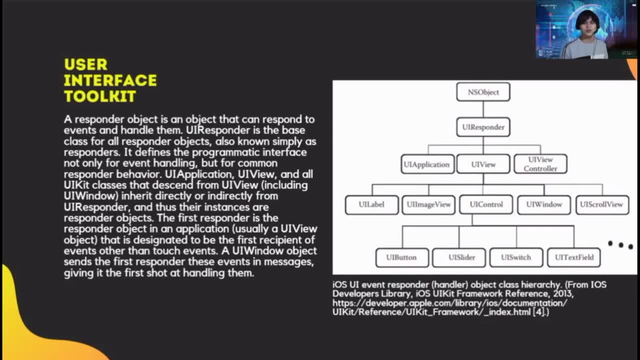 So UI application, UI view and all UI kit classes that descend from UI view, including UI window, inherit directly or indirectly from UI responder And thus their instances are responder objects. The first responder is the responder object in an application. 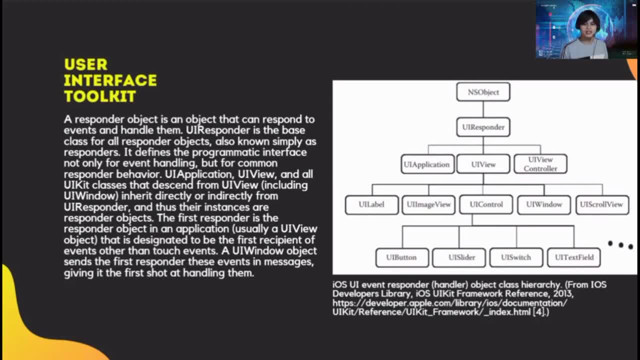 Usually a UI view object that is designated to be the first recipient of events other than touch events. So a UI window object sends the first responder these events in messages, giving it to the first shot at handling them. Okay so, inanak nanggakay tabo sila nanggakommunicate, communicate, rin na sila. 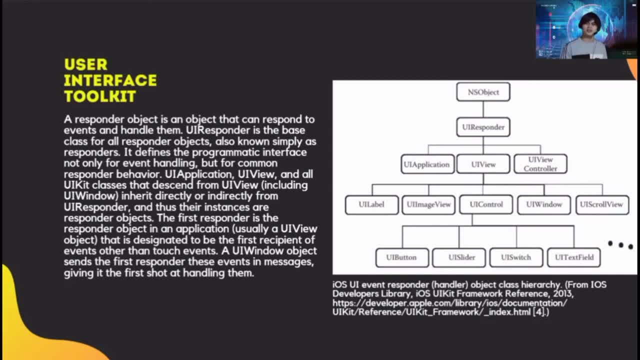 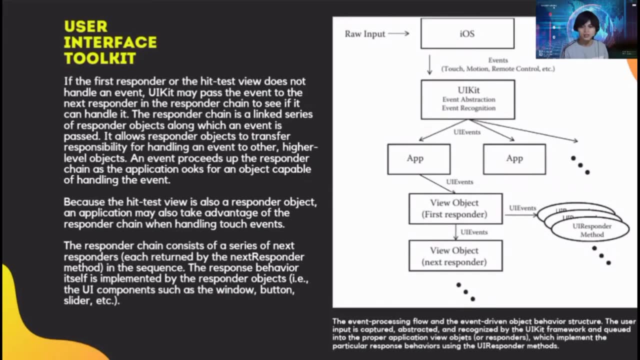 There's an object, there's a responder and the responder And the responder, will you know, siya mag-respond if there are something that need to be processed. Okay, Yun, Okay, So this is the last one, I think. 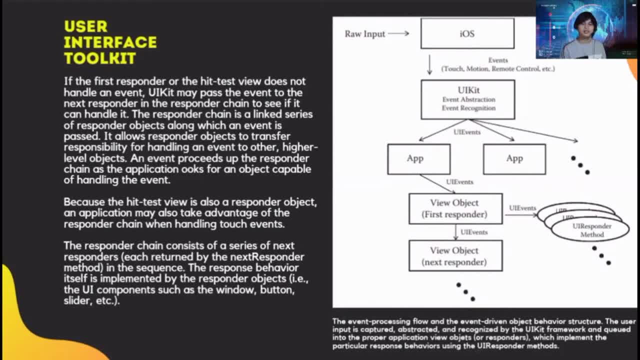 So in this diagram, if the first responder, di ba siya mag-lantaw or the hit test view, does not handle an event, UI kit may pass the event to the next responder. So the next responder in the responder chain to see if it can handle it. 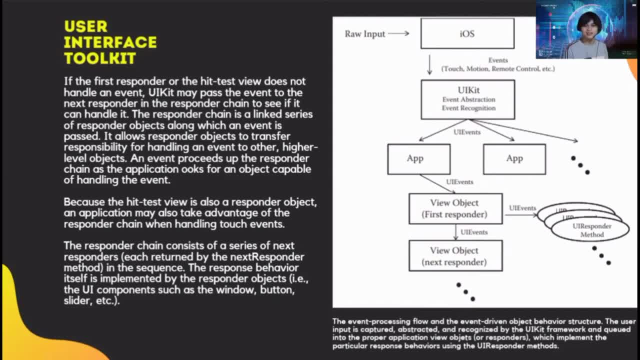 Okay, So the responder chain is a link series of responder objects along with an event is passed. It allows responder objects to transfer responsibility for handling an event to other higher level objects. Okay, So an event proceeds up the responder chain as the application loads. 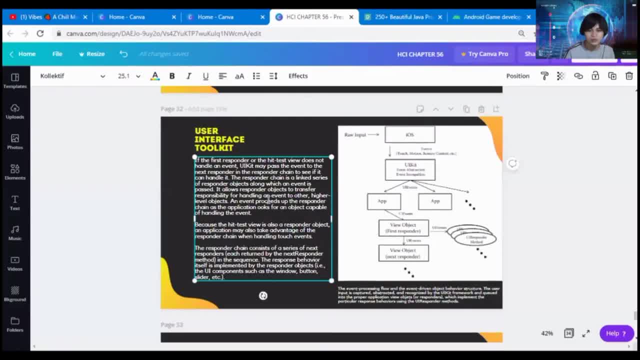 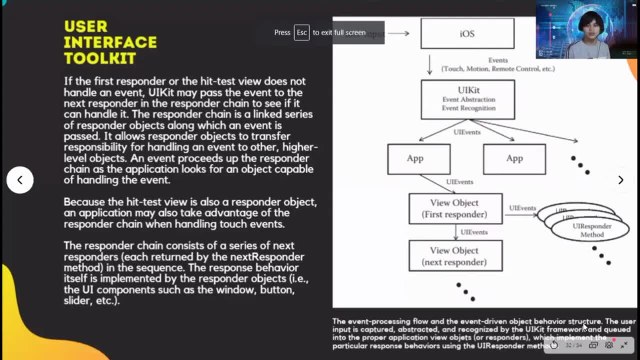 So the next responder chain looks: oh sorry guys. application looks for an object capable of handling the event And because the hit test view is also a responder object, an application may also take advantage of the responder chain when handling touch events. 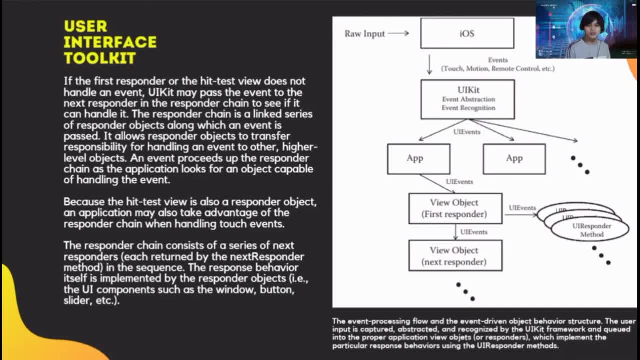 So the responder chain consists of a series of next responders. It's returned by the next responder, It's returned by the next responder method in the sequence. So the response behavior itself is implemented by the responder objects or the UI components, such as the window button slider. 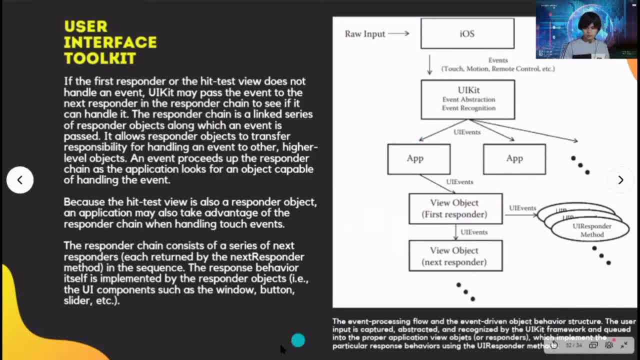 Okay, So this one is example. So this is the event processing flow Flow, Event processing flow of the event-driven object behavior structure. Okay, So the user input is captured and then abstracted. Okay, Okay, Okay. 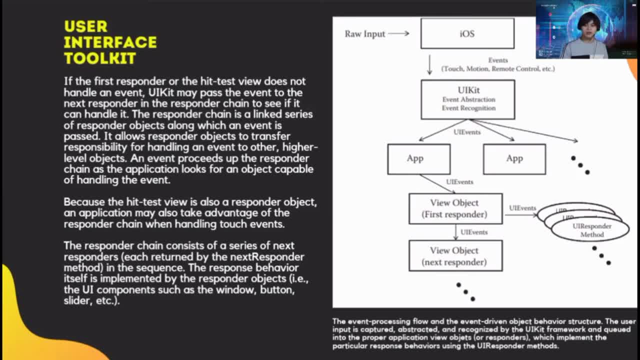 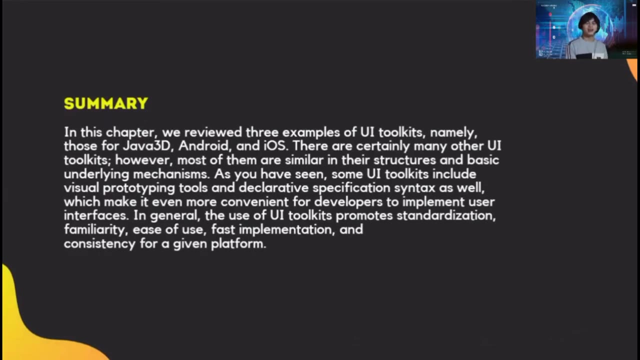 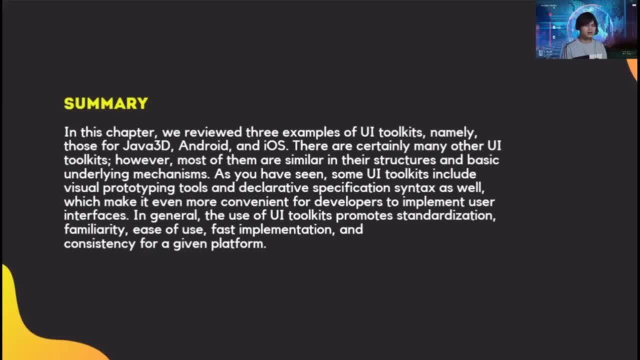 Okay, I hope that you get the point. you get some, some basic idea on how the developers create an application called a code nation using the different programming languages. so because I gotta the logic- are the same. no, there is an event handler, there is an event listeners and there are different. 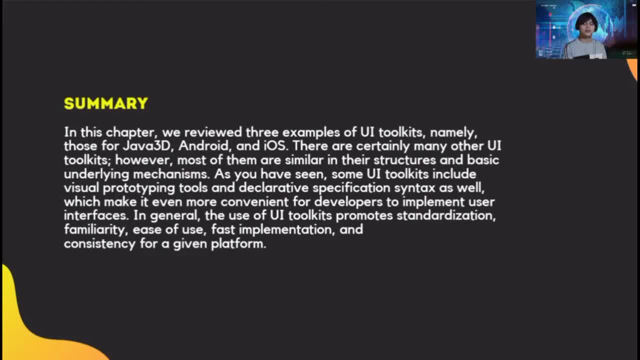 callback methods, callback functions that the developers use. no, there are different libraries. pretty fine, now the meter no longer my callback functions for you to be able to, you know, produce an output or process. concern was a process, okay. so in this chapter we reviewed three examples of a UI toolkits. we have Java 3d or the. 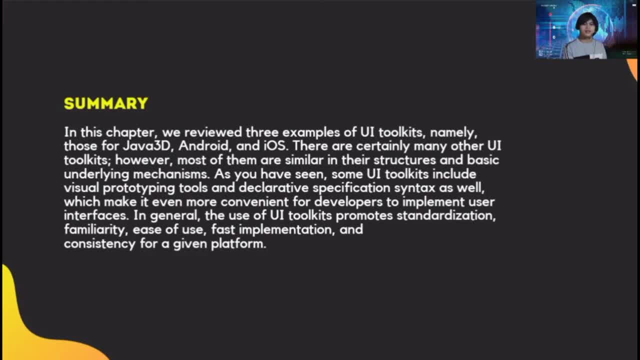 Java actually Java out, and then the Android and iOS. so there are certainly many other UI toolkits again that can go. however, most of them are similar in their structures and basic underlying mechanism. okay, like a ratio, see those names in the methods. no logic, but the same one as Ellah Kongun. I don't say okay, so as you have, 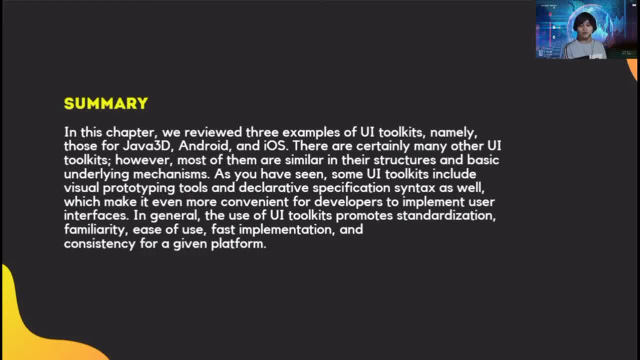 seen. some UI toolkits include visual prototyping tools and declarative specification syntax, which means that it does not actually document the it even more convenient for developers to implement user interfaces. so in general, the use of ui toolkits promotes standardization, familiarity, ease of use, fast implementation and consistency of 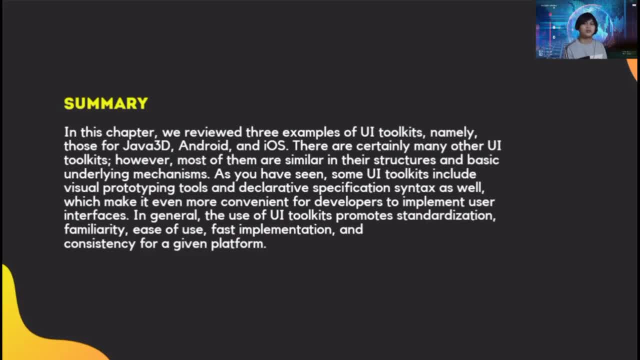 a given platform, so it's very important that you have, that you use a different, that you use a toolkit now when creating program, because it would be very hard for you to display a button, inputs, um image, dialogues- if there is no toolkits. okay, so more on asia, guys, um, in order for you to develop. 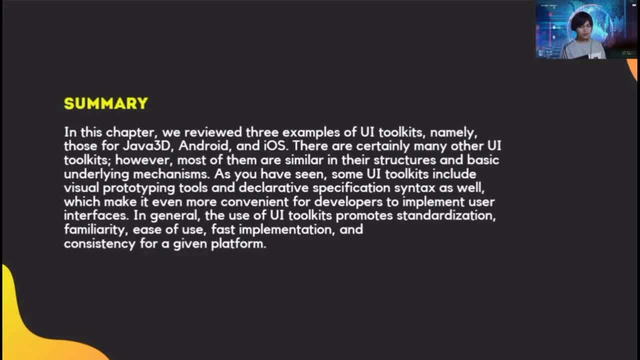 a really great, great system. okay, so it's very important now in in hci, you should know that user interface ux ui designs, and then you should know that user interface is one of the most important tools in our company. okay, so i hope that you've learned something. if there are things that um not clear to you and